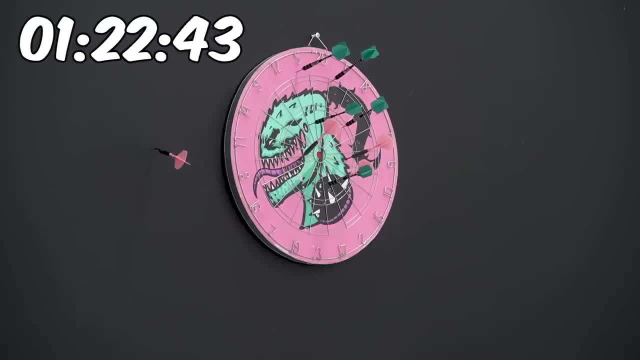 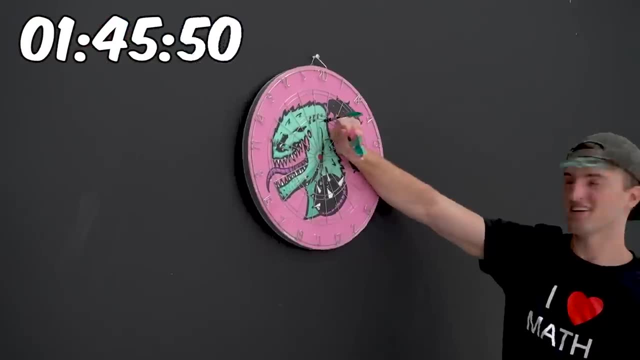 Zach, you better hurry. Michelle, how do you do a 100-digit math problem that fast? It's just progressively getting worse. Okay, I'm going to Hail Mary this. No, Jake, move, move, move, Hurry. 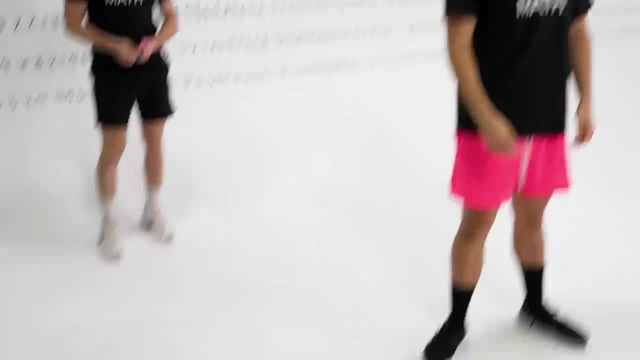 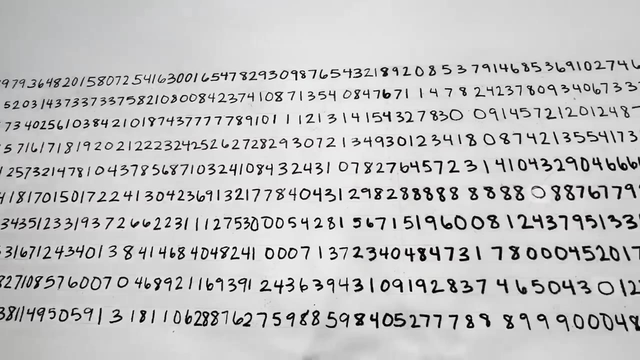 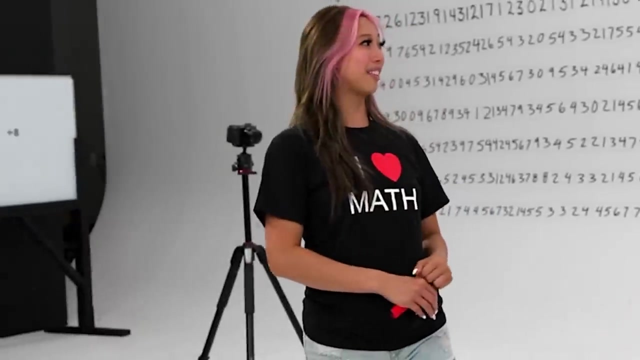 Stop Correct. Oh my goodness, He didn't hit a bullseye. I don't get paid enough for this. You don't get paid at all. On the floor is a 1,000-digit math problem, And if my boyfriend and videographer can finish that giant slice of pizza before I solve this, they win a grand. 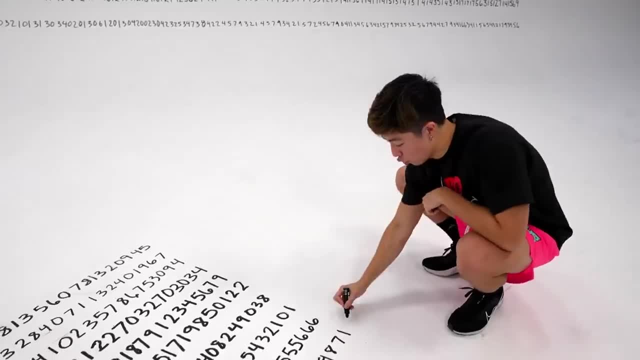 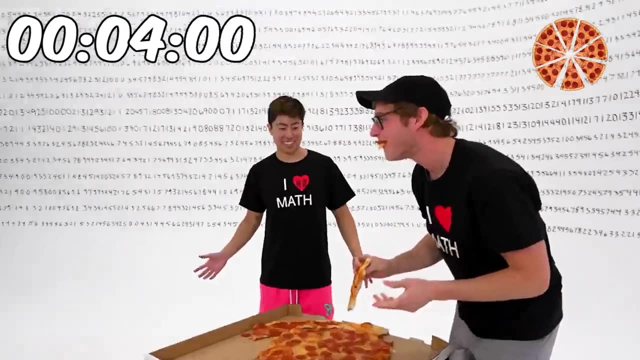 Good, I'm starving. Okay, Zach, write a number that I can divide by. I think a tricky number would be seven. Go, Does anyone have a napkin? I can hear David chewing and it's so gross You're touching everything. 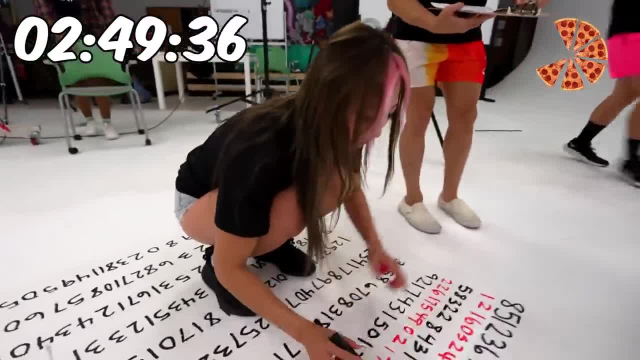 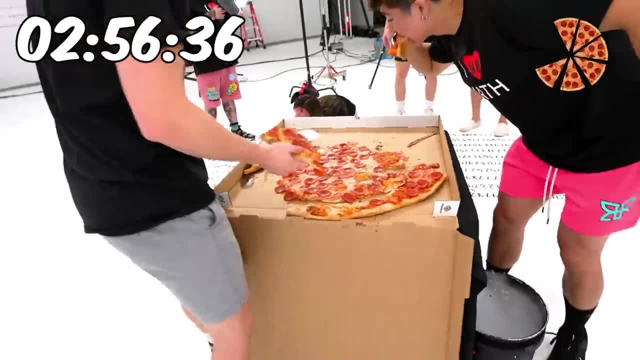 How am I supposed to eat this? I'm going to eat this whole pizza. I am not giving a grand up to David. What are you doing? Zach's eating with a fork and a knife, so it's going to go a little bit slower. 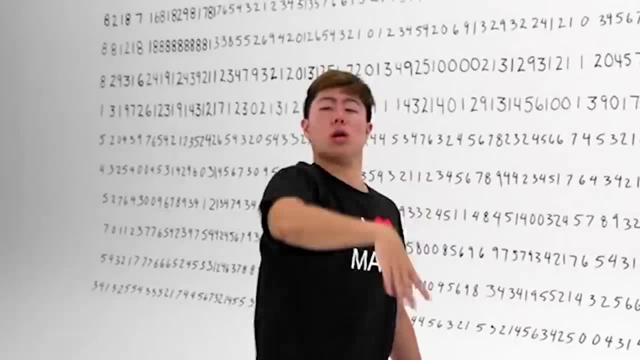 That's 200 digits down. Wait, David, I feel kind of queasy. Good job, Michelle. I feel so much better now I don't feel any better. You're almost halfway through. Put that down. We need to take a break and regroup here. 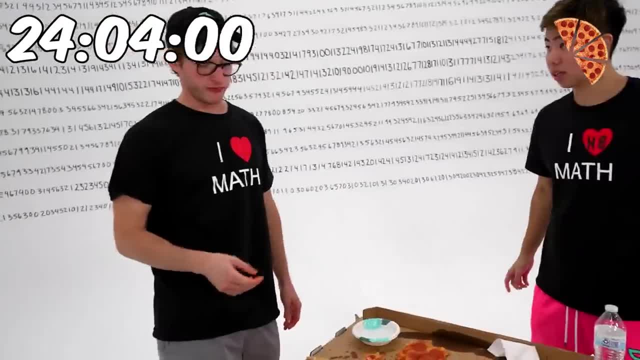 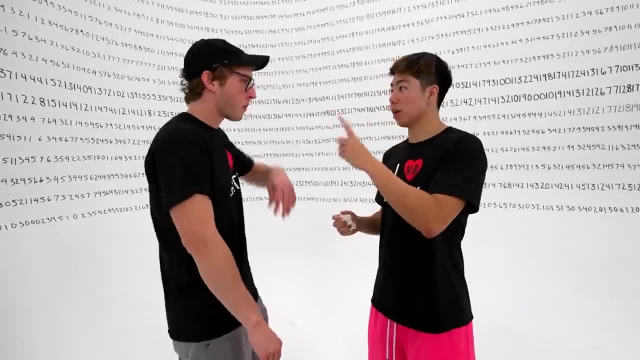 Four, seven, one, six. All right, just finish. I don't know if this is worth $1,000.. I'm going to throw it. I have to leave. So in the back we actually have smoothie blender. 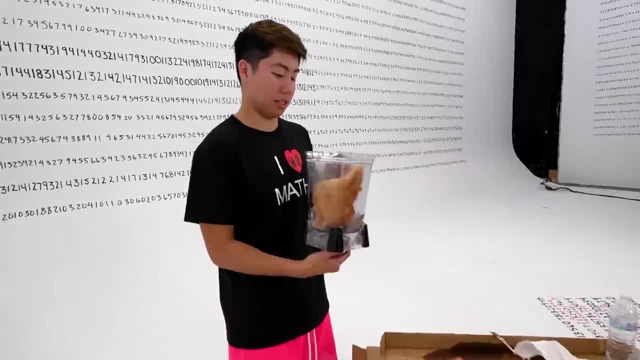 Yes, What we can do is we can put water inside, We can put pizza inside, Swirl it up and then you can drink it. because I'm not drinking that, Sure, that's fine. Ew, I can't believe he's actually doing it. 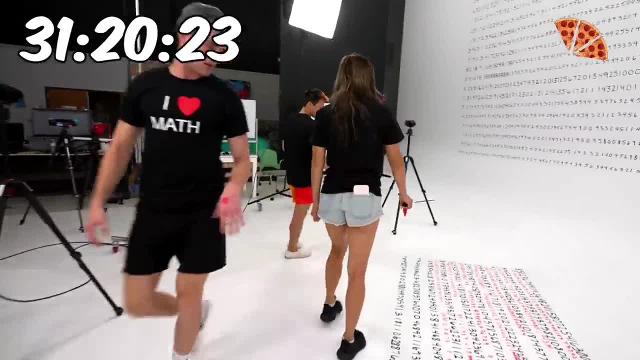 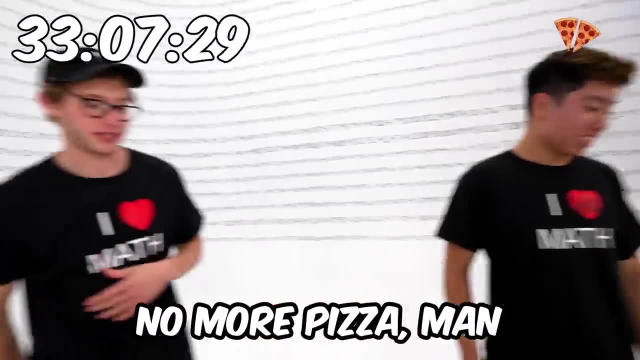 I can't do it with him distracting me. Three more lines, 300 more numbers. All right, David, just focus one bit at a time. Two, six, two, nine, two, No more pizza, No more pizza, no. 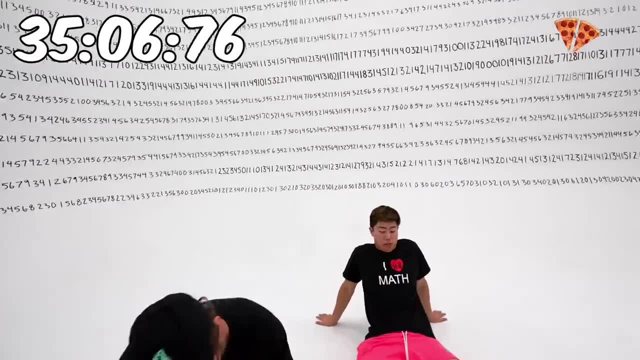 I think the plan is we sit down for a moment and when Michelle's on the last line, we go hard. He's got almost 100 digits, 100 digits to go. You guys are done. 100 digits left. Last row: Michelle. 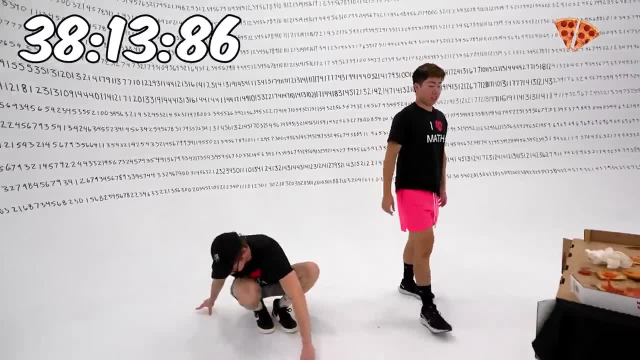 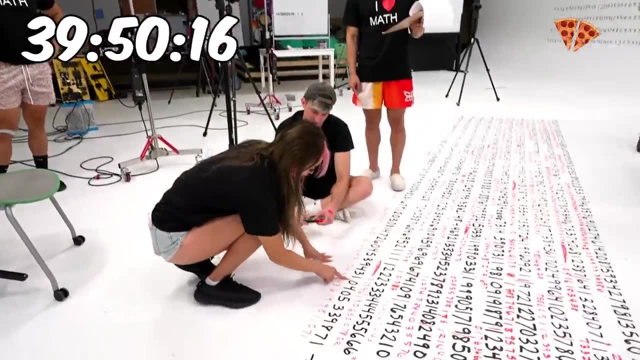 Let's go. 100 digits left. 100 digits left. Last row: 100 digits left. All right, let's finish strong. I am the pizza man. Wait 4, 4,, 9,, 8,, 1.5.. 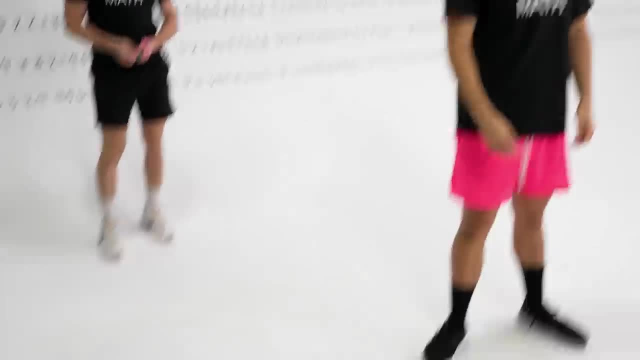 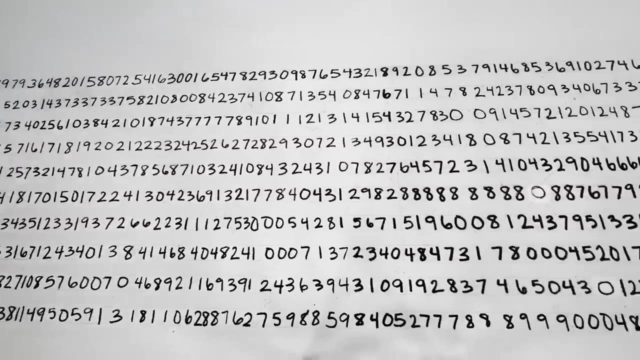 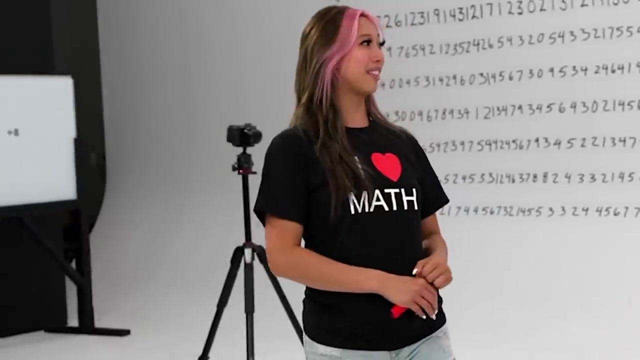 Stop Correct. Oh my goodness, He didn't hit a bullseye. I don't get paid enough for this. You don't get paid at all. On the floor is a 1,000-digit math problem, And if my boyfriend and videographer can finish that giant slice of pizza before I solve this, they win a grand. 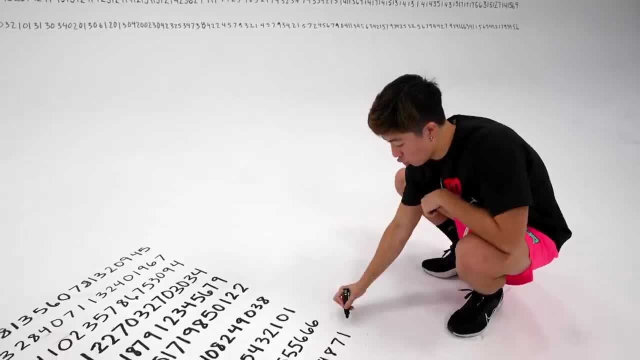 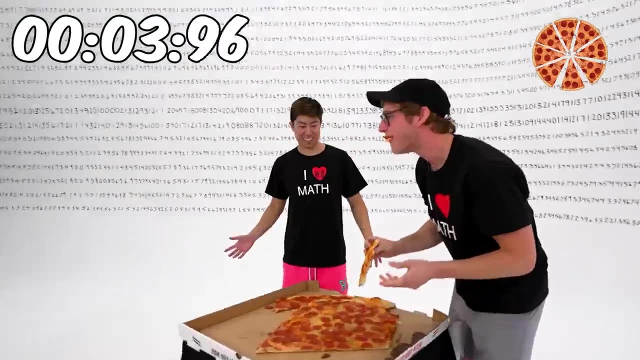 Good, I'm starving. Okay, Zach, write a number that I can divide by. I think a tricky number would be seven. Go, Does anyone have a napkin? I can hear David chewing and it's so gross You're touching everything. 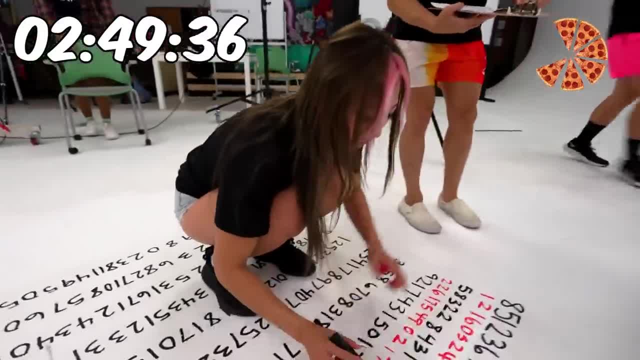 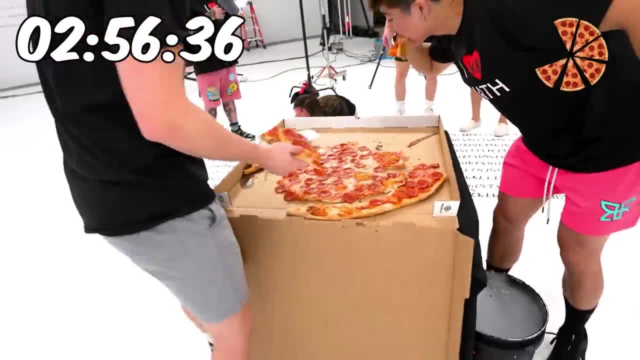 How am I supposed to eat this? I'm going to eat this whole pizza. I am not giving a grand up to David. What are you doing? Zach's eating with a fork and a knife, so it's going to go a little bit slower. 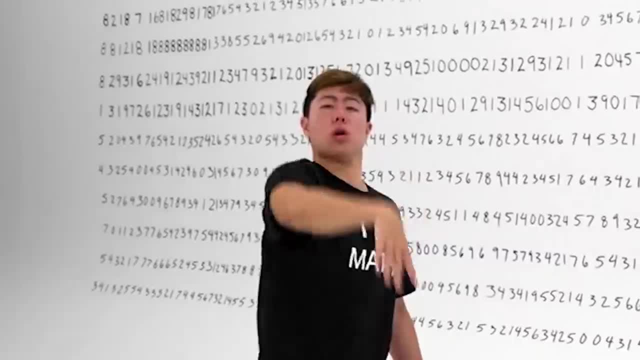 That's 200 digits down. Wait, David, I feel kind of queasy. Good job, Michelle. I feel so much better now I don't feel any better. You're almost halfway through. Put that down. We need to take a break and regroup here. 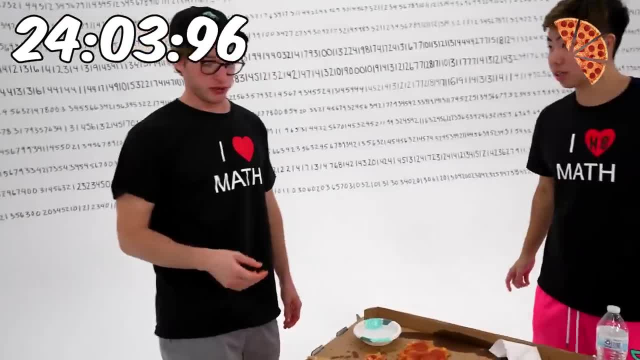 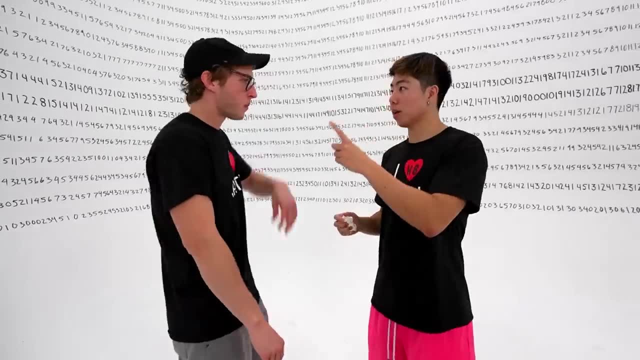 Four, seven, one, six, All right, just for this. I don't know if this is worth $1,000.. Uh-huh, uh-huh, I'm going to throw up. I have to leave. So in the back we actually have a smoothie blender. 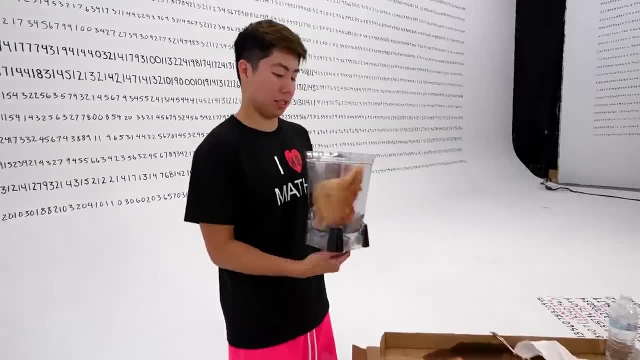 Yes, What we can do is we can put water inside, we can put pizza inside, Swirl it up and then you can drink it. because I'm not drinking that, Sure, that's fine. Ew, I can't believe he's actually doing it. 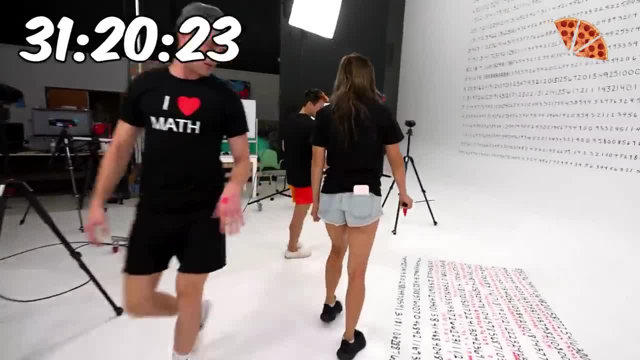 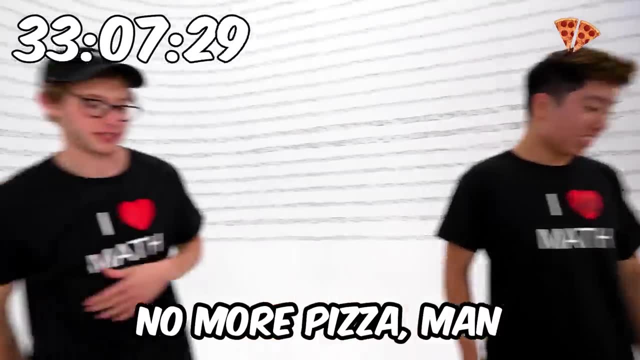 I can't do it with him distracting me. Three more lines, 300 more numbers. All right, David, just focus one bit at a time. Two, six, two, nine, two, No more pizza, No more pizza, no. 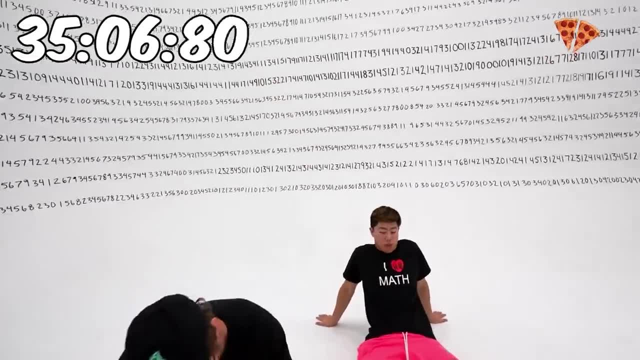 I think the plan is we sit down for a moment and when Michelle's on the last line, we go hard. He's got almost 100 digits, 100 digits to go. You guys are done. 100 digits left. Last row: Michelle, let's go. 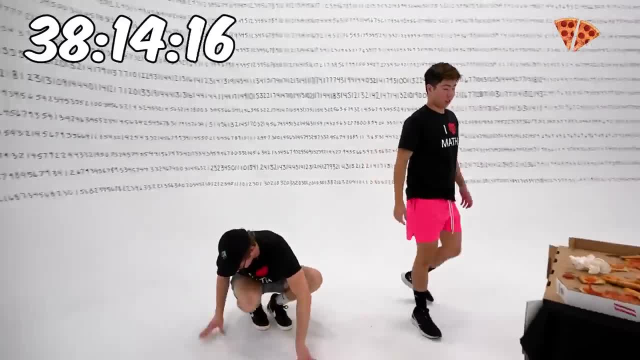 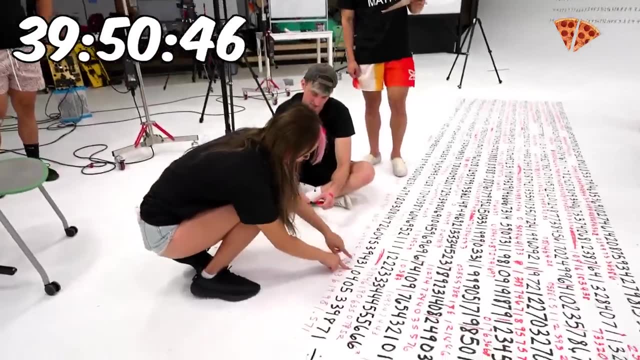 100 digits left. 100 digits left Last row: 100 digits left. All right, let's finish strong. I am the pizza man. Wait. 4,, 4,, 9,, 8,, 1.5.. 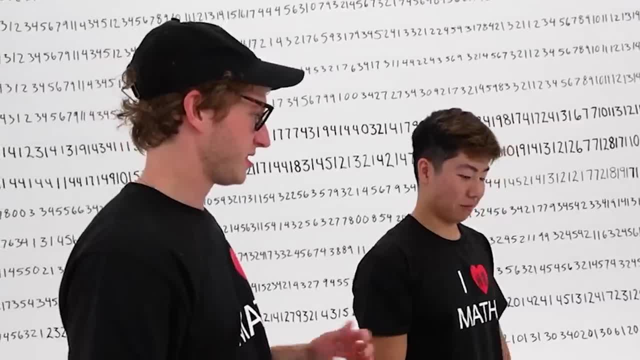 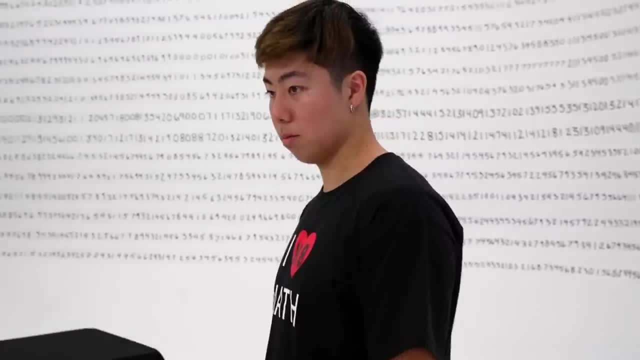 Yes, I hate pizza. Hey man, I was going to eat that. If you pause right here, my answer should match this, which is the right answer. Are you ready for the 10,000?? I'm not ready. Have fun with that. 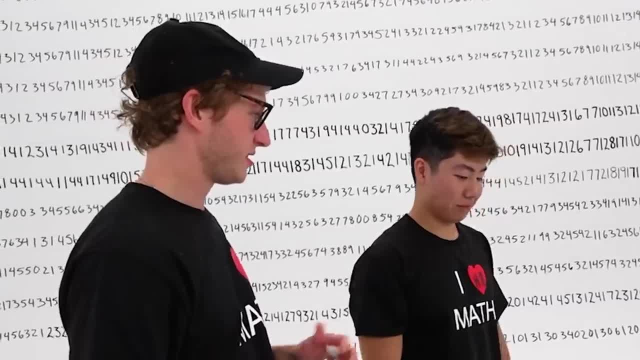 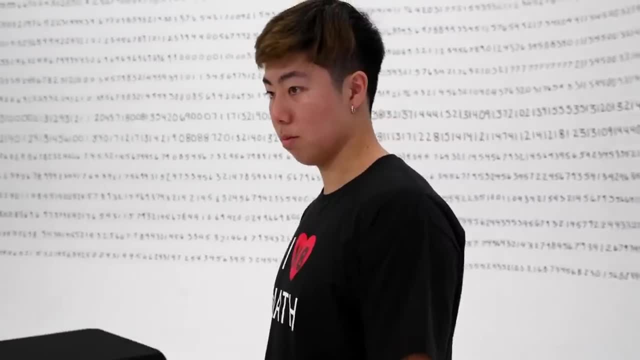 Yes, I hate pizza. Hey man, I was going to eat that. If you pause right here, my answer should match this, which is the right answer. Are you ready for the 10,000?? I'm not ready. Have fun with that. 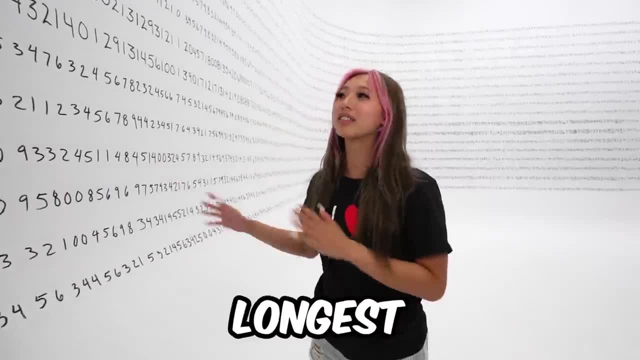 I'm scared. I'm scared to do the 10,000.. I need a poop now. This is the world's longest math problem. This math problem is so big we had to fill up this entire wall and we didn't have enough. 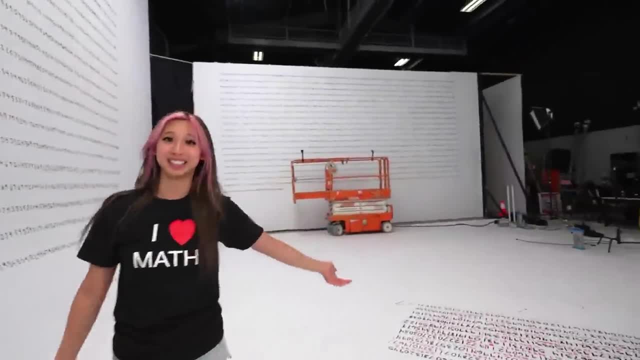 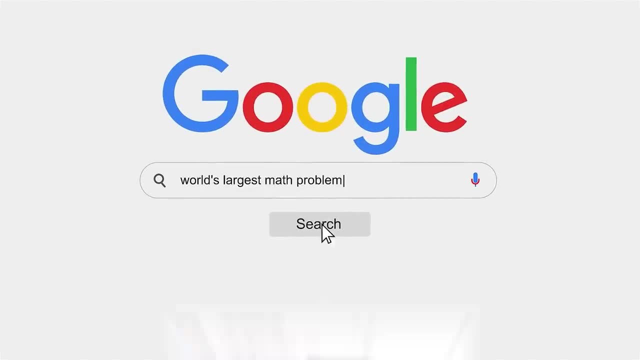 space. so we had to fill up an extra wall just to fit 10,000 digits, And I'm using a scissor lift because this math problem is too tall. My team and I have done weeks of research and we saw that the world's longest math problem. 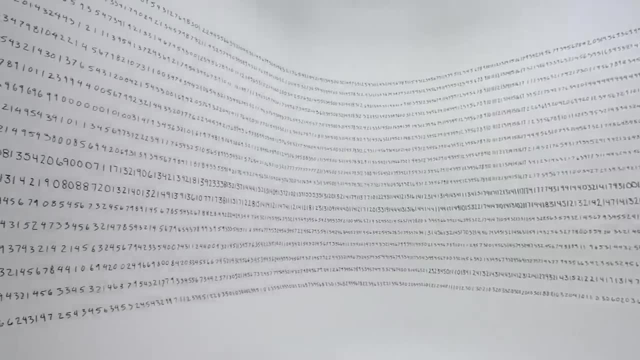 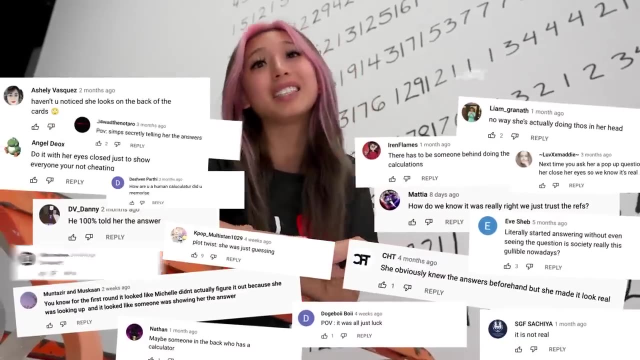 is a proof, but that's a little bit different and I've never seen a 10,000-digit problem like this. I don't even know if I can do this. Hey, Look at those boobs. I love this problem. I've seen a lot of comments saying that this is fake, but this is not fake and I'm going. 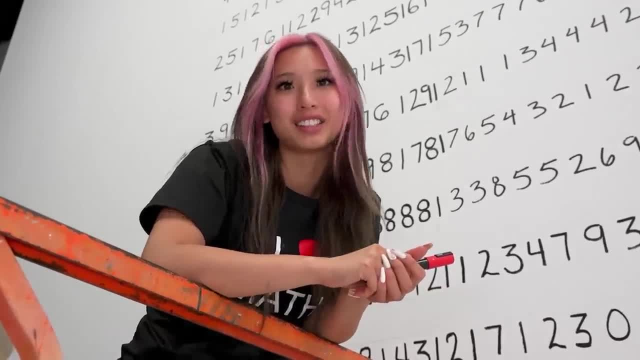 to prove it, because there's no way I can memorize 10,000 digits. Let's do this. I'm so scared of heights. This is really wobbly, Zachary. I don't even know what. I'm dividing it by. 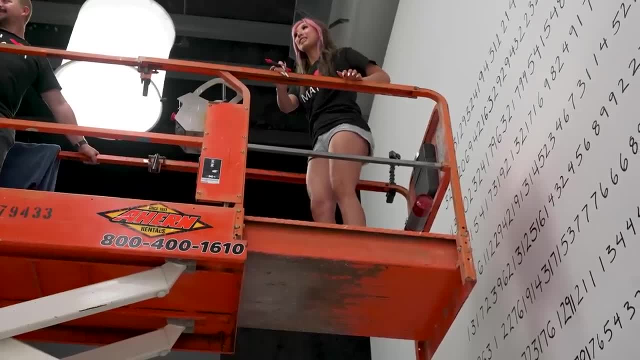 Zach, give me a number. All right, Six-a-roonie Okay. Seven, six, eight. No way she can actually do this. This is ridiculous. Zero six. I need to find a number. I need to find a number. 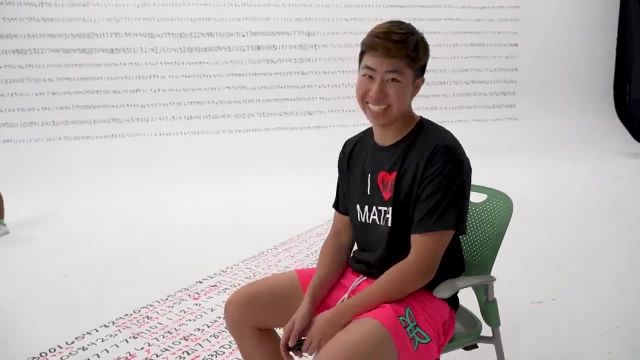 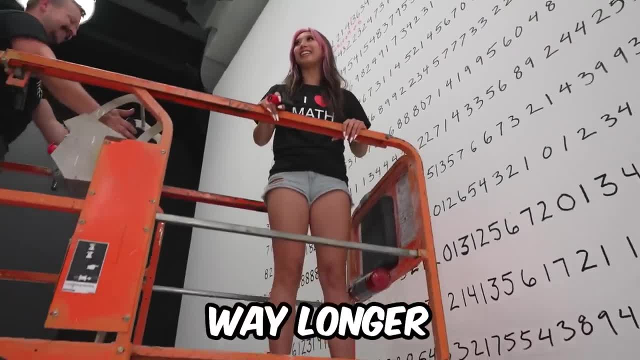 I need to find a number- Yes, six. I need to move. I have to go down, move and then go back up again. This is going to take way longer than six hours. Don't be so funny. I'm in the middle of this shoot. 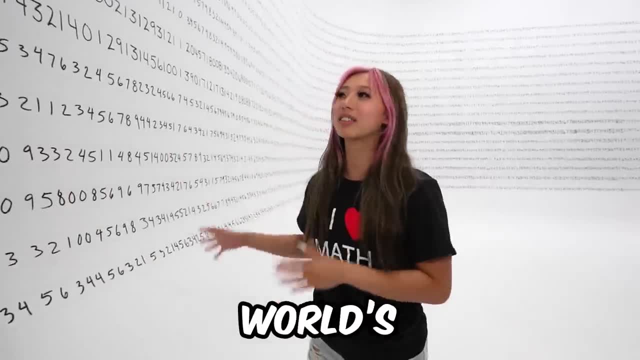 I'm scared. I'm scared to do the 10,000.. I need a poop now. This is the world's longest math problem. This math problem is so big we had to fill up this entire wall and we didn't have enough. 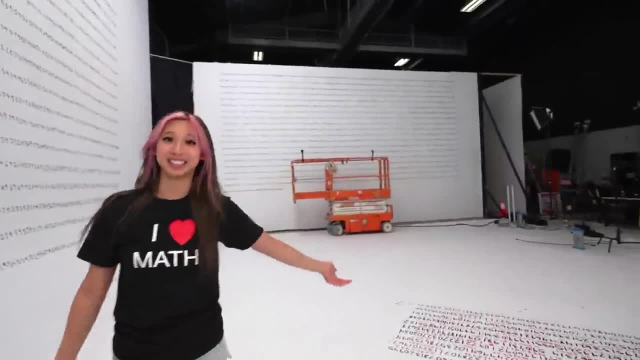 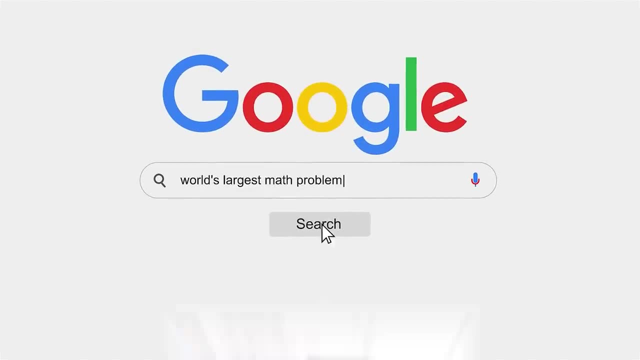 space. so we had to fill up an extra wall just to fit 10,000 digits, And I'm using a scissor lift because this math problem is too tall. My team and I have done weeks of research and we saw that the world's longest math problem. 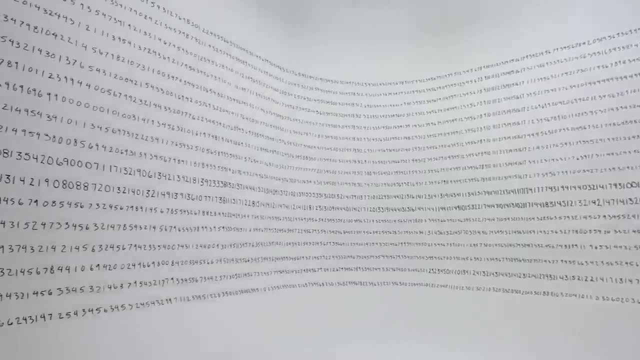 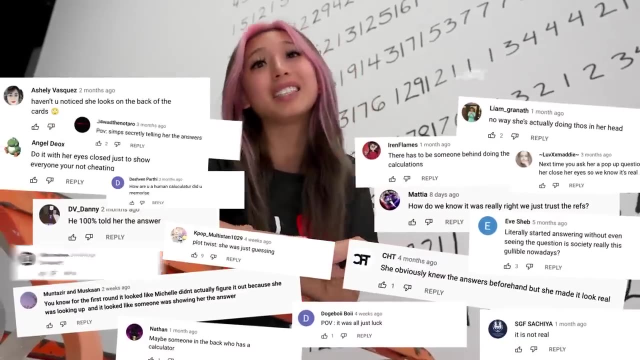 is a proof, but that's a little bit different and I've never seen a 10,000-digit problem like this. I don't even know if I can do this. Hey, It even says boobs. I love this problem. I've seen a lot of comments saying that this is fake, but this is not fake and I'm going. 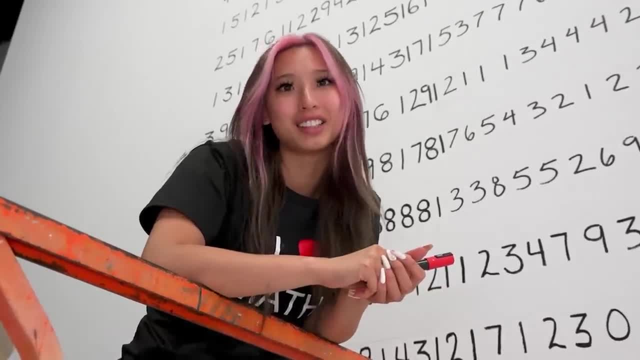 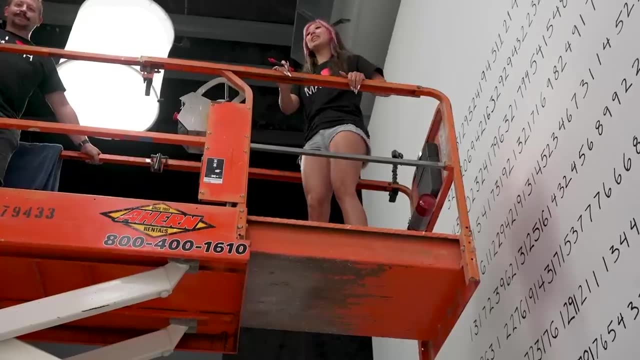 to prove it, because there's no way I can memorize 10,000 digits. Let's do this. I'm so scared of heights. This is really wobbly, Zachary. I don't even know what. I'm dividing it by. 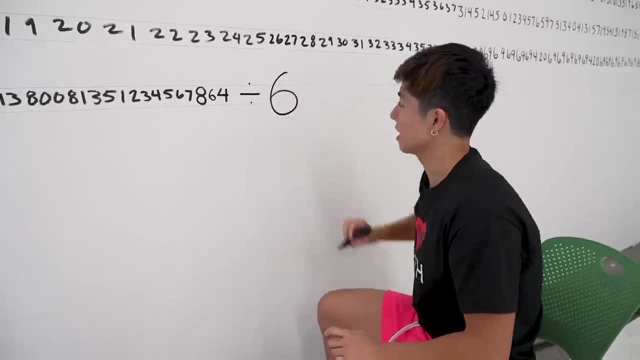 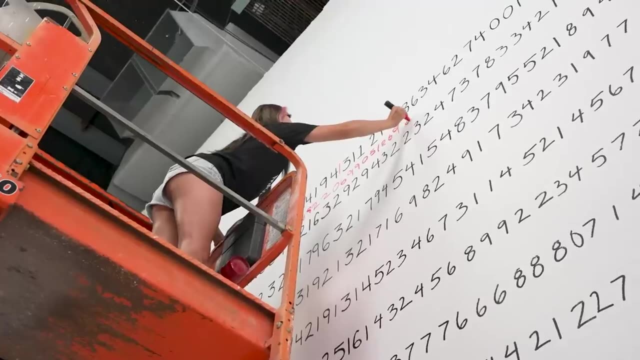 Zach, give me a number. All right, Six-a-roonie, Okay. Seven, six, eight. No way she can actually do this. This is ridiculous. Two zero six Eight. I need to move. I have to go down, move and then go back up again. 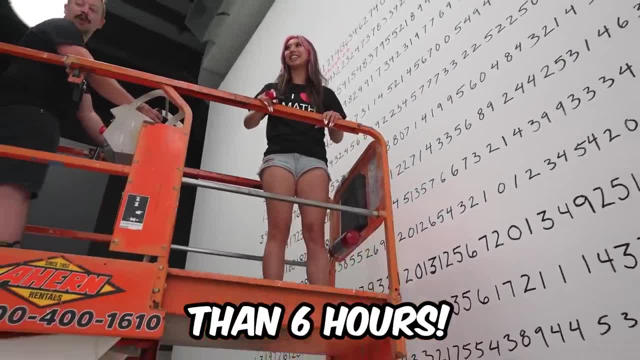 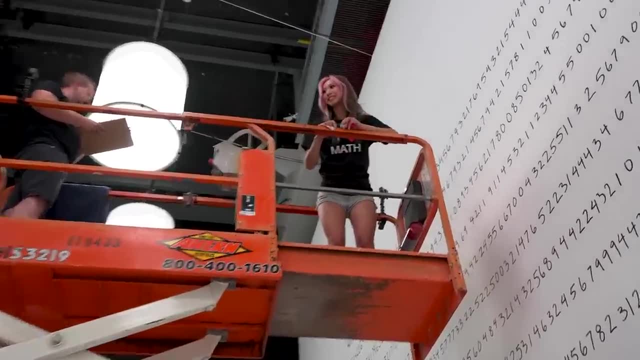 This is going to take way longer than six hours. Don't be so funny if in the middle of the shoot, the scissor lift breaks. Zachary, every time I get a number wrong, I get pelted with water balloons. Okay, 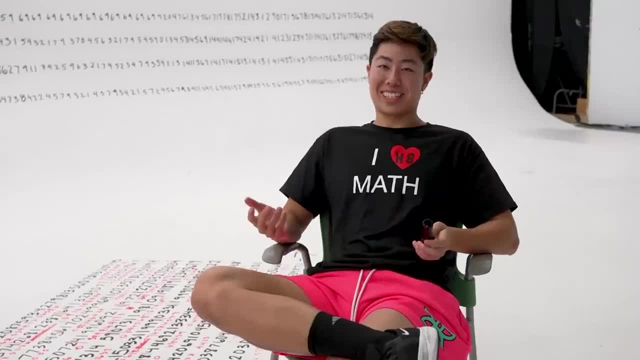 I can do that. I'm not going to get any wrong. I'm doing well. There's 10,000 digits. She's going to get one wrong: Four, two, seven, nine. I'm feeling very confident right now. 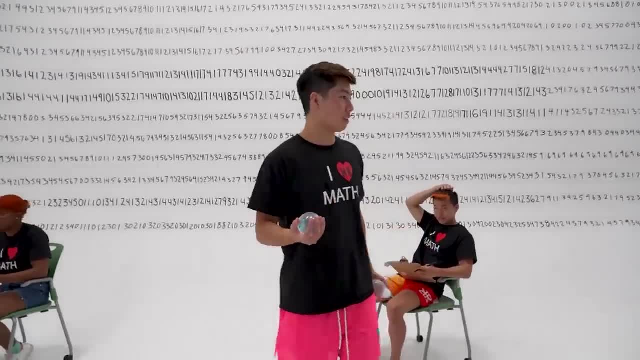 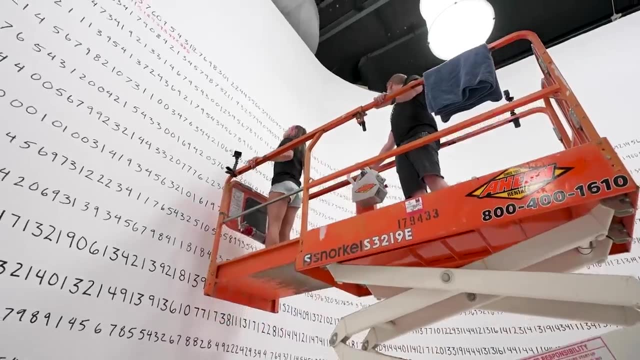 I'm not getting any of them wrong. Am I allowed to just pelt her for no reason? One eight nine, three eight five. One six, three, eight zero, nine, two, four. When is she going to get one wrong? 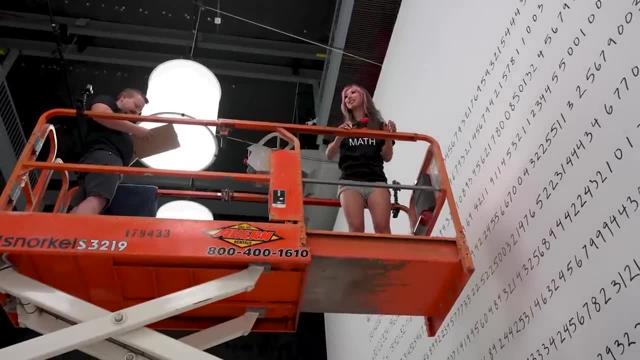 The scissor lift breaks. Zachary, every time I get a number wrong, I get pelted with water balloons. Okay, I can do that. I'm not going to get any wrong. I'm doing well. There's 10,000 digits. 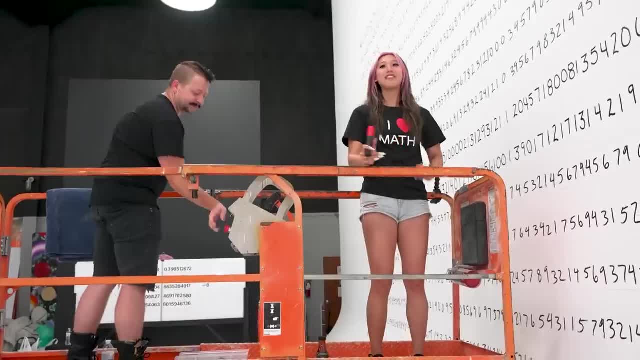 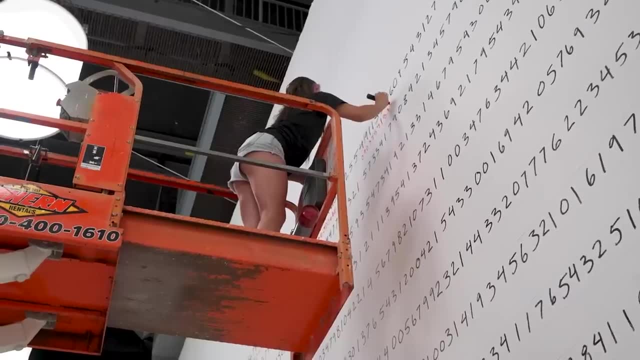 She's going to get one wrong, Four, two, seven, nine. I'm feeling very confident right now. I'm not getting any of them wrong. Am I allowed to just pelt her for no reason? 1, 8,, 9,, 3, 8, 5. 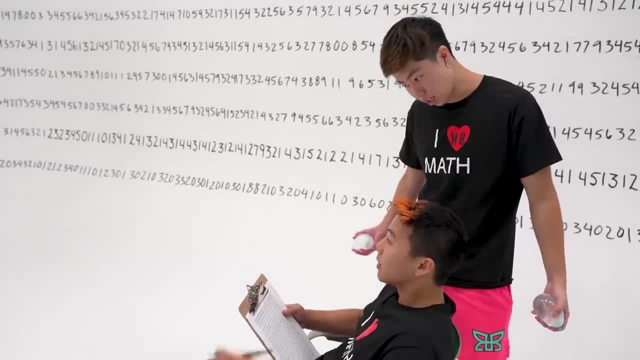 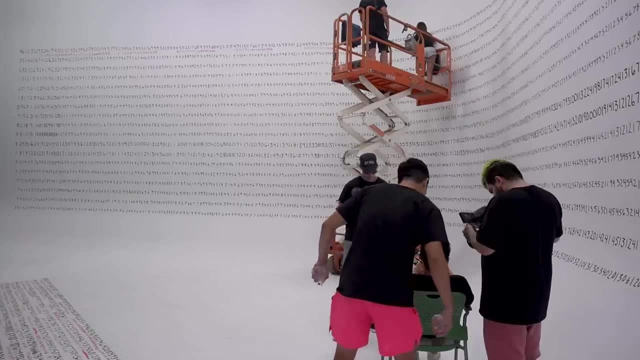 1,, 6,, 3,, 8,, 0,, 9, 2. When's she gonna get one wrong? She always clutch when there's pressure. 8,, 8,, 5,, 7, 5- What was that? What was that? 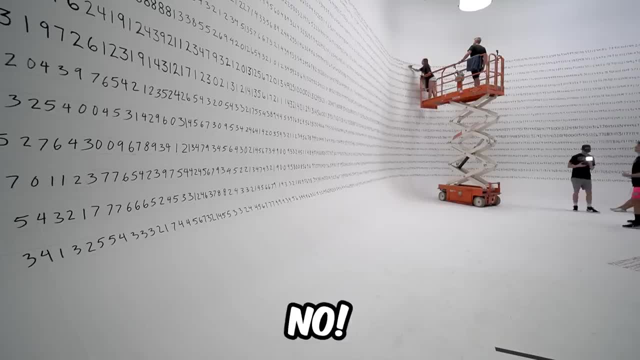 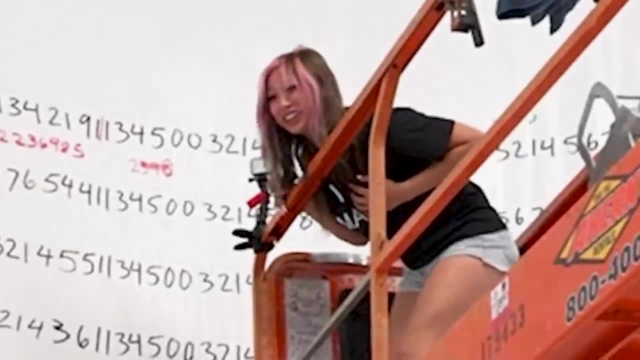 Wait, what was it? 2- Wait, you said 5, right, No, 6!, I'm at 6!. Wait, no, Alright, I'm at You. hit my boob After that. I'm never getting another one wrong. 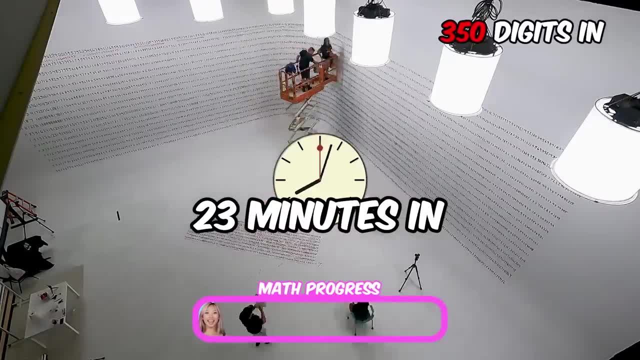 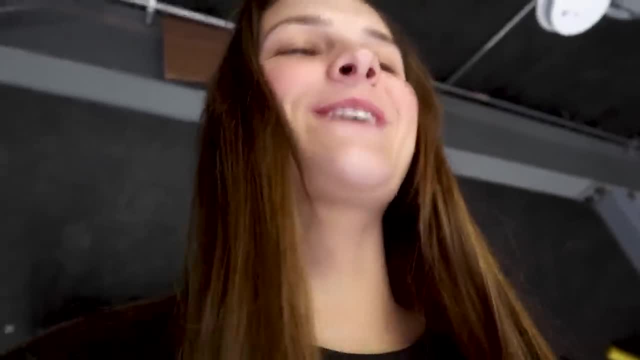 I'm feeling really confident. I went through the first line pretty fast. 18 more lines to go, plus the wall: 0, 5, 3, 5. Michelle, can you mess one up so I can throw a water balloon at you? No, thank you. 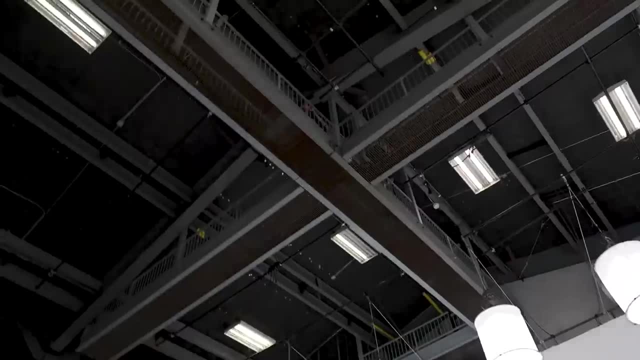 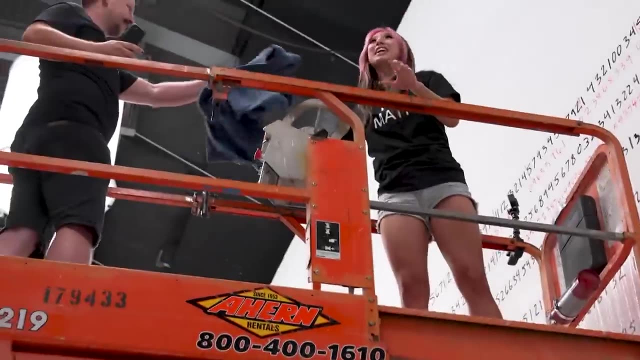 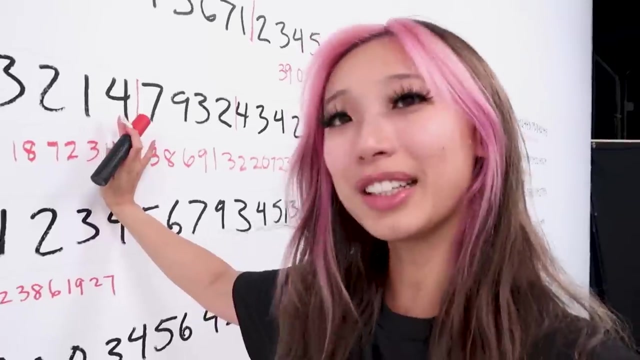 9, 4. You can't see. No, I forgot a zero. My problem: I did less than a dollar, I did a thousand digits And I'm sick and tired of this math problem. I just want to show you guys why I put like a little dash here. 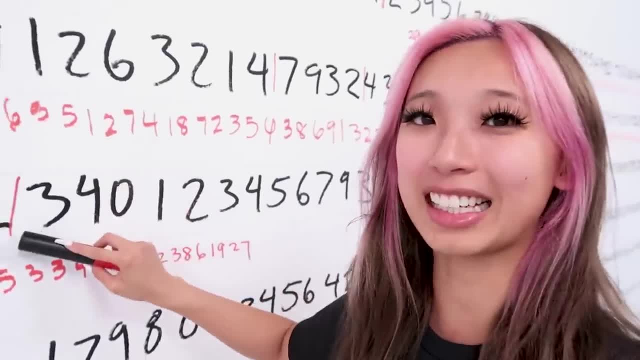 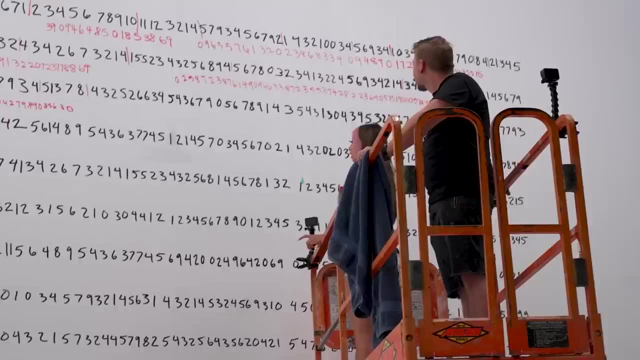 But every time there's a dash that means there's a zero. Then it helps me keep track. in case I make a mistake, I can go back to where this little checkpoint is Alright. so Michelle's been working on the problem for around an hour. I have an idea to mess with her a little bit. 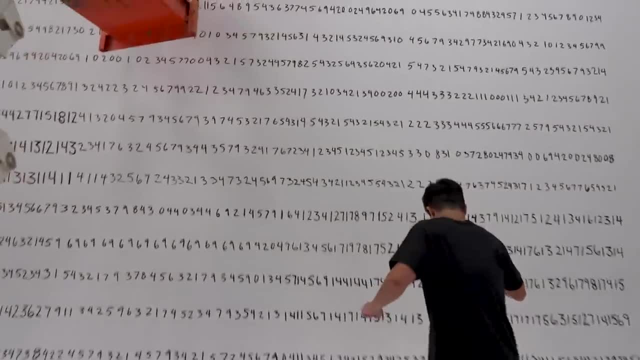 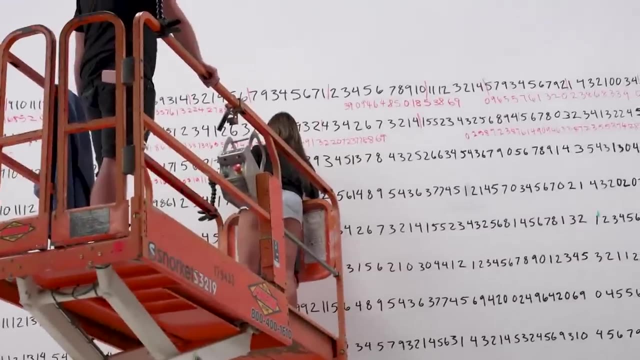 I'm gonna write a random letter somewhere And see if that messes her up later on in the video. 3,, 4,, 7, 2: You're doing well so far, Michelle. You're doing very well indeed. 8,, 9,, 7, 1. 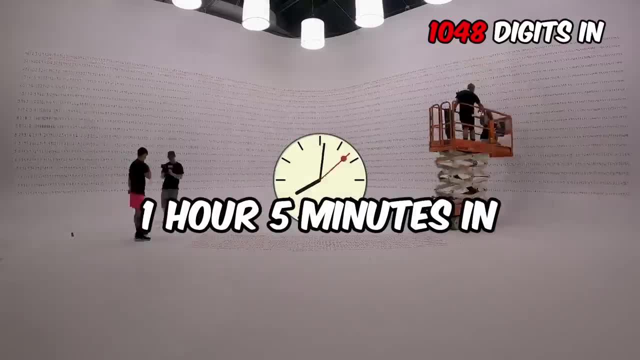 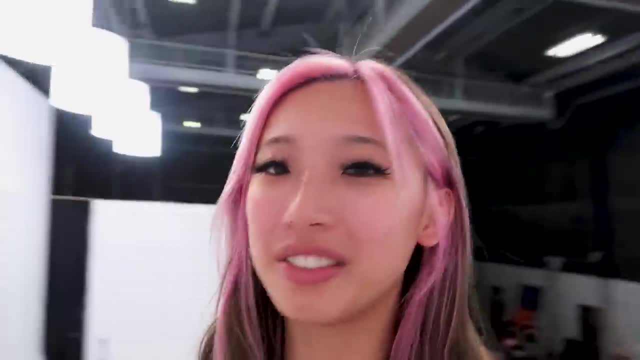 Alright, just finished the last digit of row 3. For those of you who are wondering how I'm getting these right, I have my team helping me check my answers. We have this super calculator that we found on the internet That helped us solve this 10,000 digit problem. 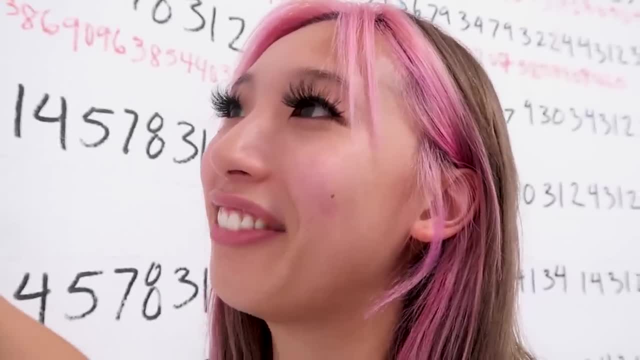 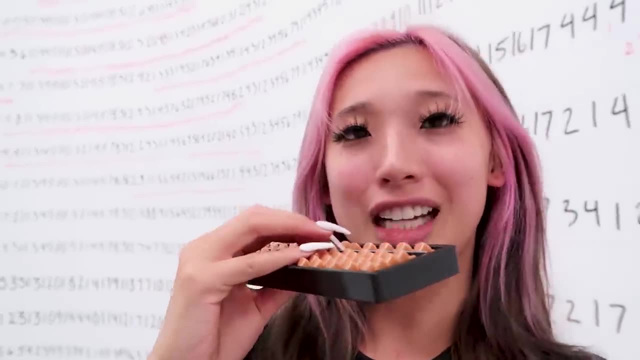 It was so scary: 9,, 5,, 5,, 7, 6. So a lot of people ask me how I'm able to do this. I use this little thing. So this is a Chinese abacus. I've been training to use this. 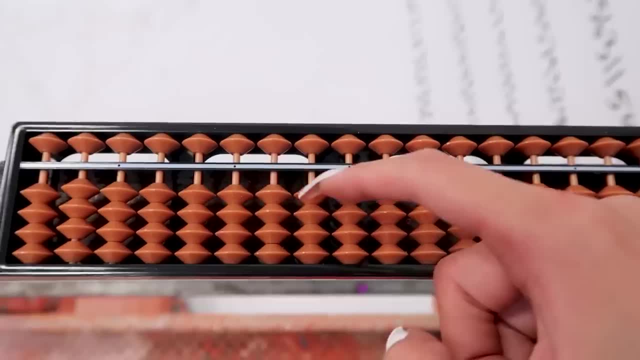 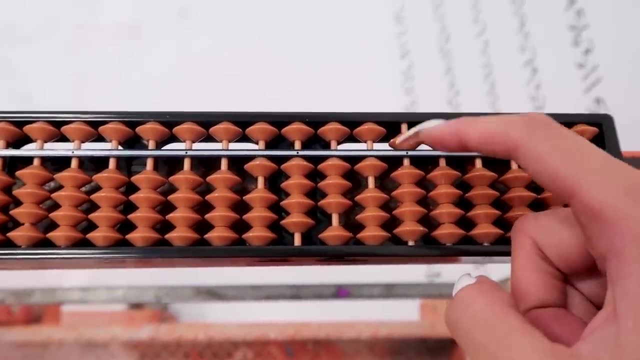 Since I was 5 years old, 1 bead is 1, 4 beads is 4, 3 beads is 3, 1, 5 And the 5 is on the top And 7 is 5 plus 2: 143,157 in my head. 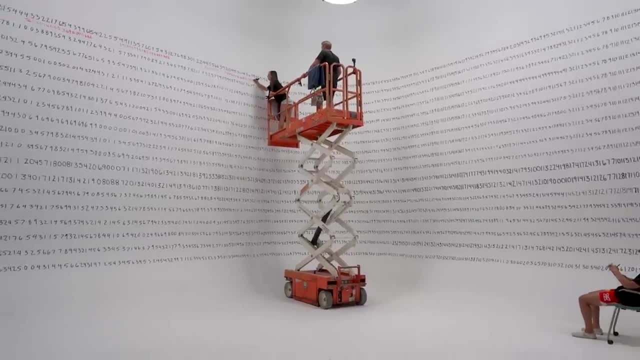 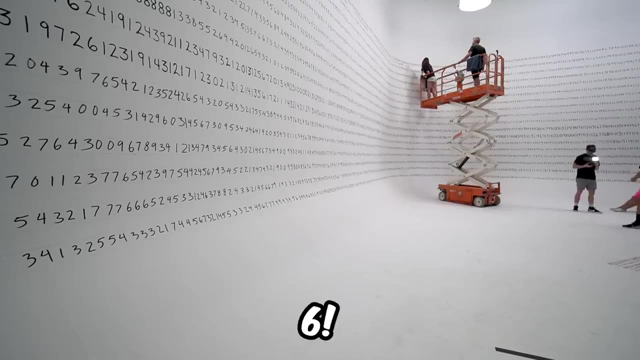 She doesn't clutch when there's pressure. Eight, eight, five, seven, five, What was that? What was that? Wait, What was it? Two? Wait, You said five, right, No Six. I'm at six. 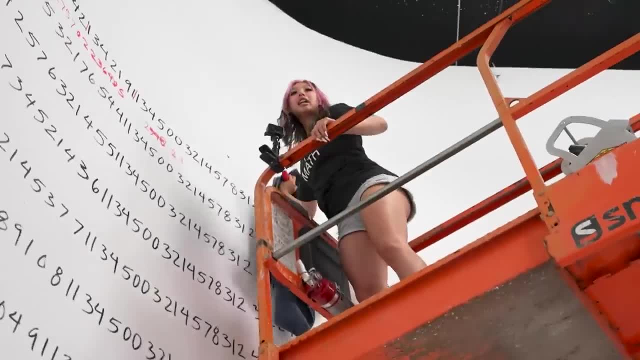 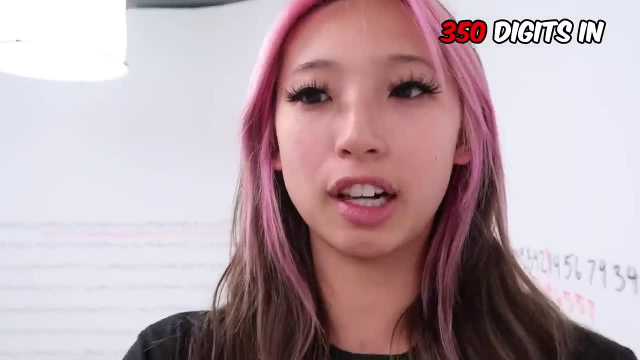 Wait, No, After that I am never getting another one wrong. I'm feeling really confident. I went through the first line pretty fast. Eighteen more lines to go, plus the wall. Zero, five, three, five. Michelle, can you mess one up so I can throw a water balloon at you? 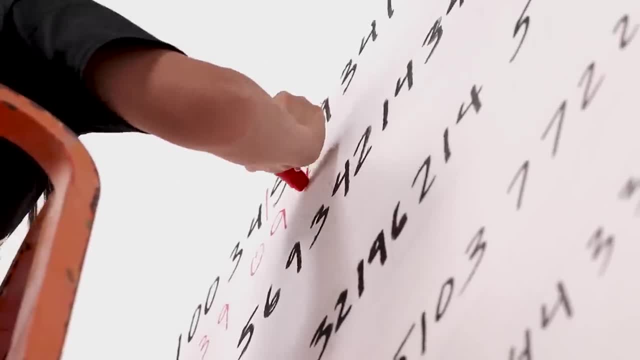 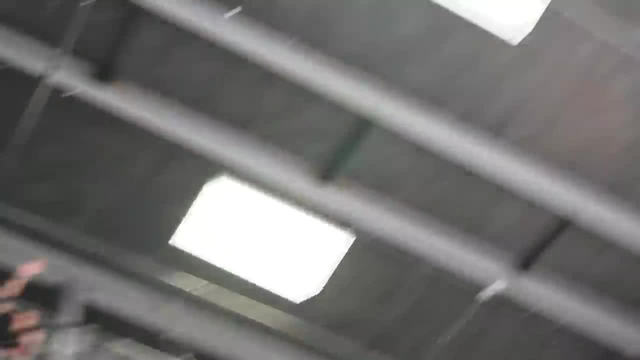 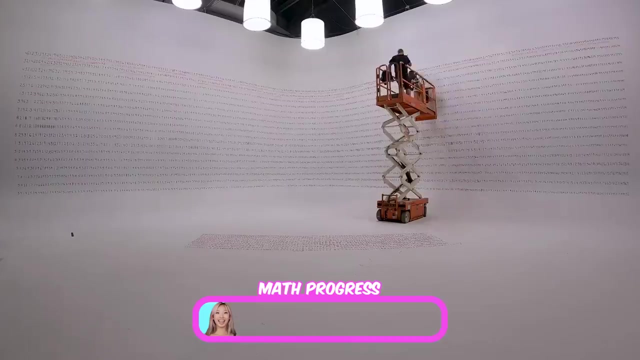 No, thank you. Nine four, I can't see. No, I forgot a zero. My problem: I did less than a thousand digits and I am sick and tired of this math problem. I just want to show you guys why I put like a little dash here. 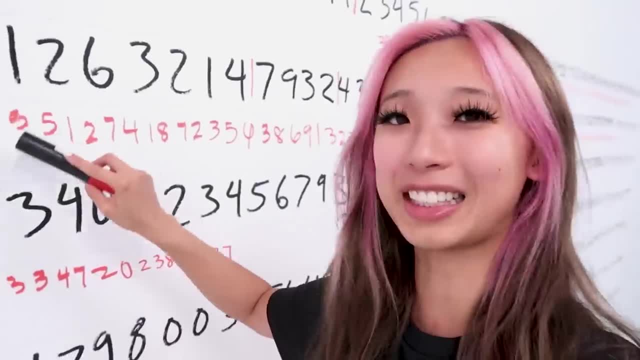 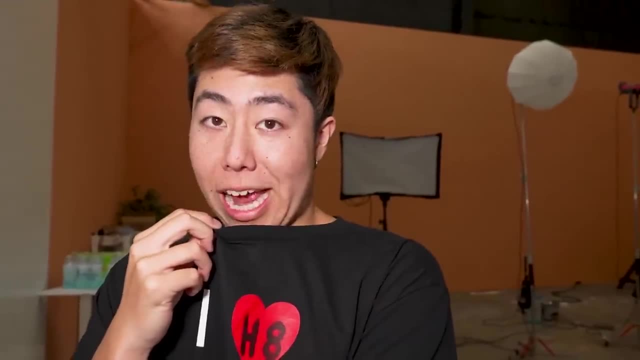 But every time there's a dash that means there's a zero. Then it helps me keep track. in case I make a mistake, I can go back to where this little checkpoint is. So Michelle's been working on the problem for around an hour. 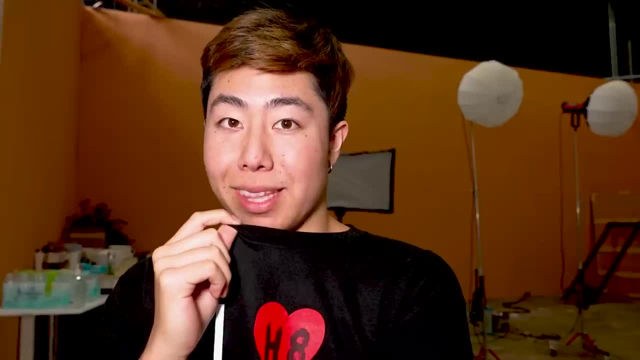 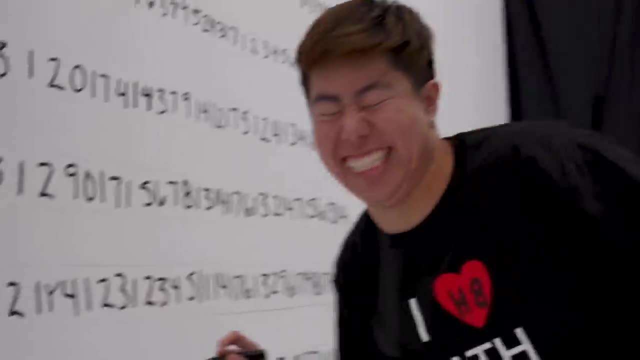 I have an idea to mess with her a little bit. I'm going to write a random letter somewhere and see if that messes her up later on in the video. Three, four, seven, two: You're doing well so far, Michelle. 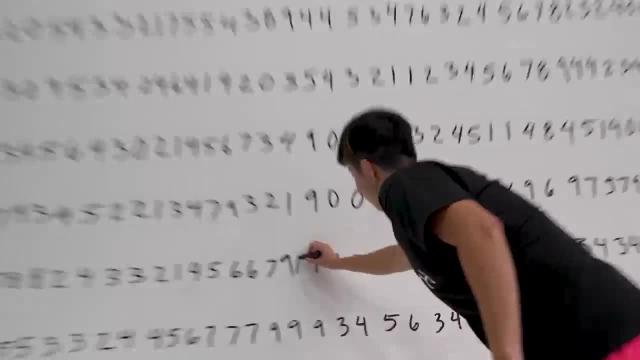 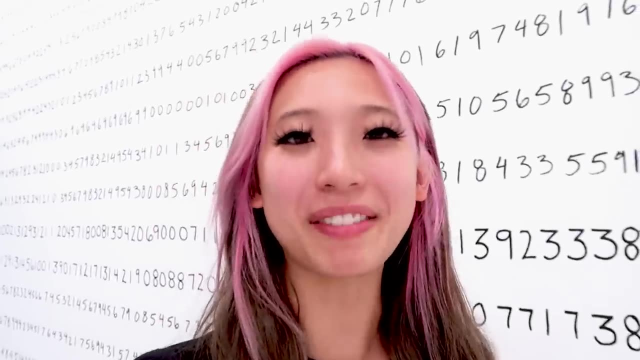 You're doing very well indeed. Eight, nine, seven, one. Alright, just finished the last digit of row three. For those of you who are wondering how I'm getting these right, I have my team helping me check my answers. We have this super calculator that we found on the internet that helped us solve this 10,000 digit problem. 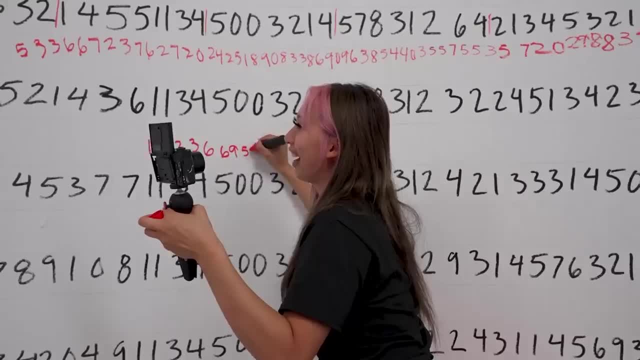 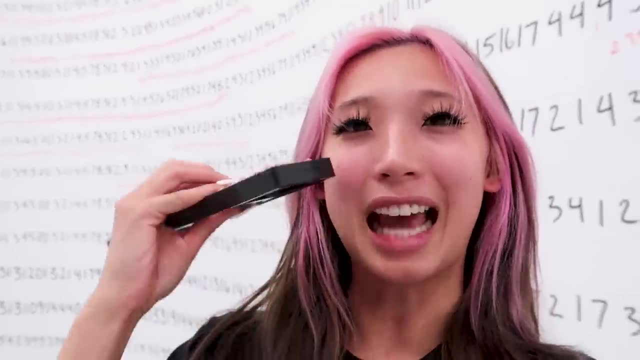 This is so scary: Nine five, five, seven, six. So a lot of people ask me how I'm able to do this. I use this little thing. So this is a Chinese advocate. I've been training to use this since I was five years old. 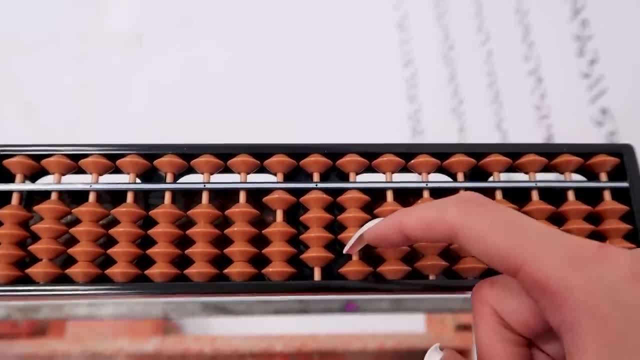 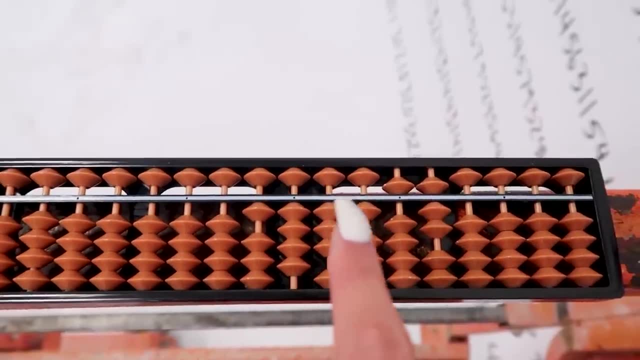 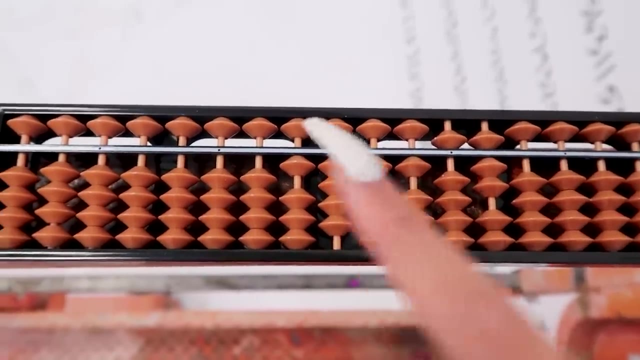 One bead is one, Four beads is four, Three beads is three, One five, And the five is on the top And seven is five plus two: 143,157 in my head. And if I want to divide by six, the only number divisible by 14 for six is two. 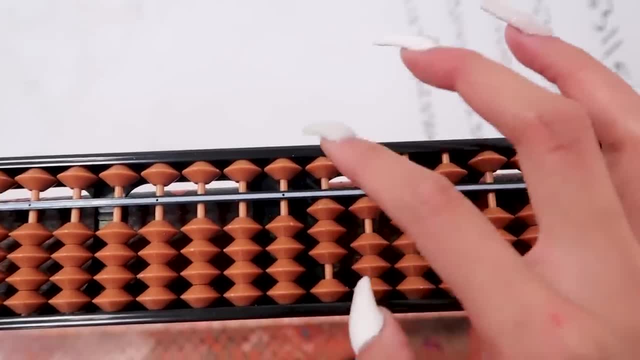 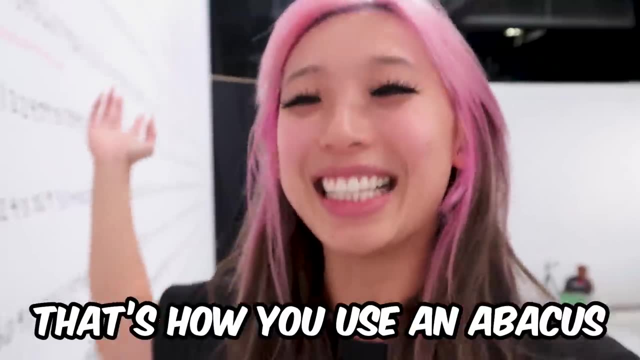 So six times two is 12.. Then three, Then eight, Then five, Then nine And five. That's how you use an advocate. Are you going to stay up here and cheer me on? No, Too many numbers, I hate math. 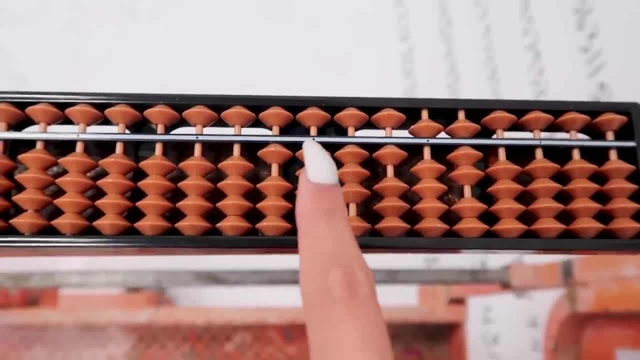 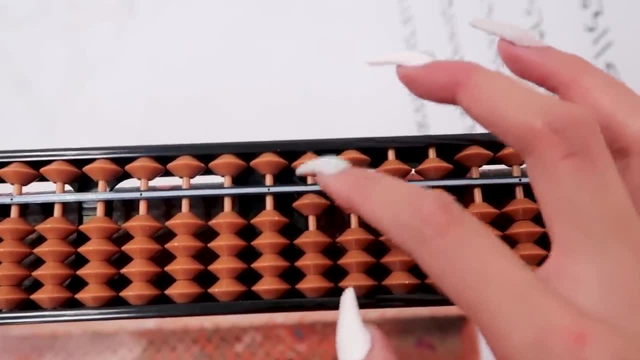 And if I want to divide by 6, The only number divisible by 14 for 6 is 2. So 6 times 2 is 12, Then 3, Then 8, Then 5, Then 9 And 5. That's how you use an abacus. 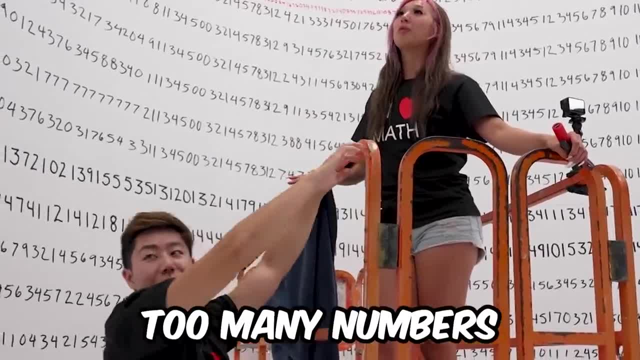 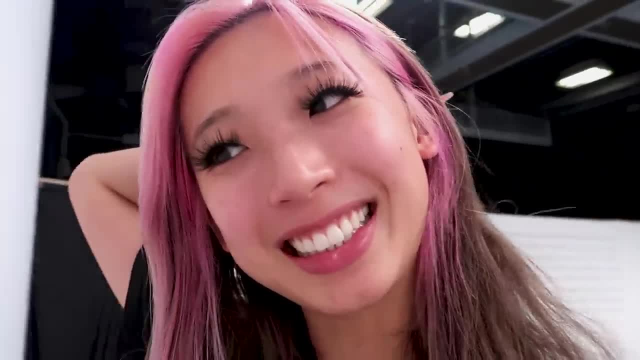 Are you going to stay up here and cheer me on? No, Too many numbers. I hate math. My brain is getting a little fried, Not going to lie. 0, 0. Kind of tired of hearing the scissor lift too. I'm not even halfway done Or even a quarter of the way done. 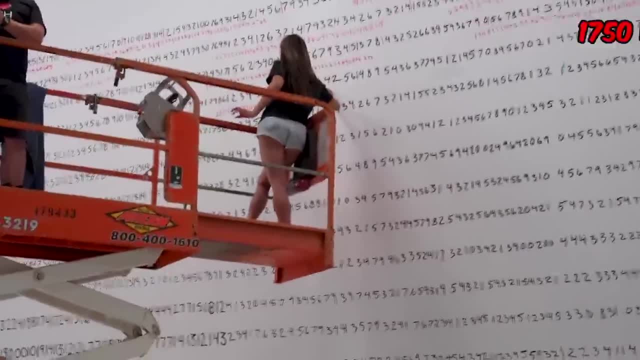 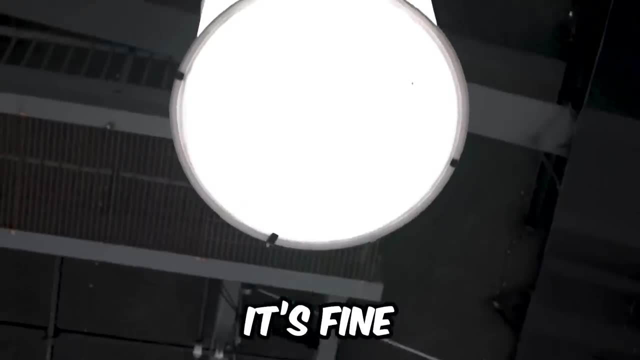 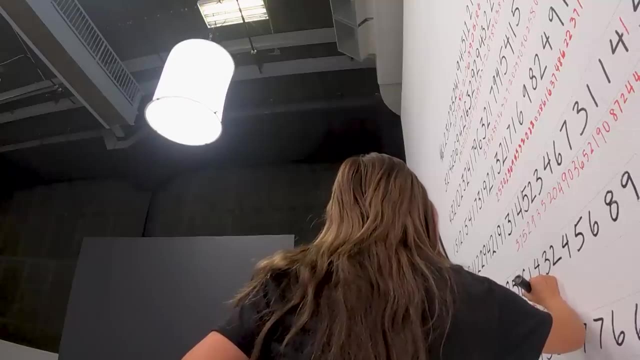 9, 6, 5, No, 6, 6. No, I caught it before anyone else did. No one cares, It's fine, it's waterproof, Mackenzie. If you hit it closely, You will see a Miss Munchie In her natural habitat. 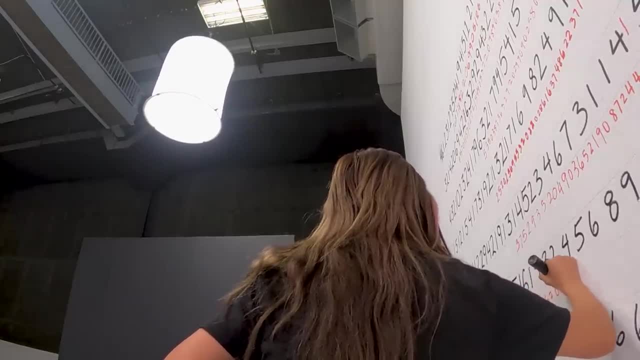 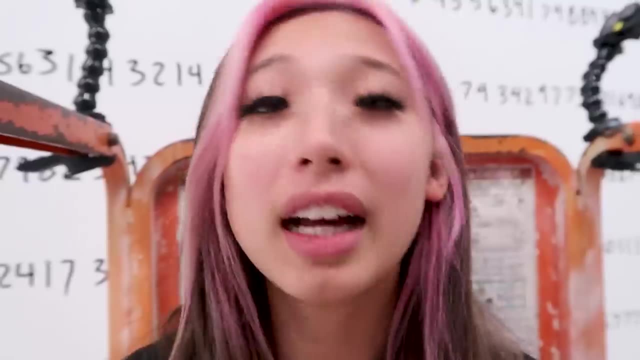 Only few species will tackle a problem. this big Thanks for watching Animal Planet, Currently 6 rows in. I don't think I feel confident about finishing by 6 hours, But I do feel confident about finishing the whole thing. So far I've only got like 4 wrong. 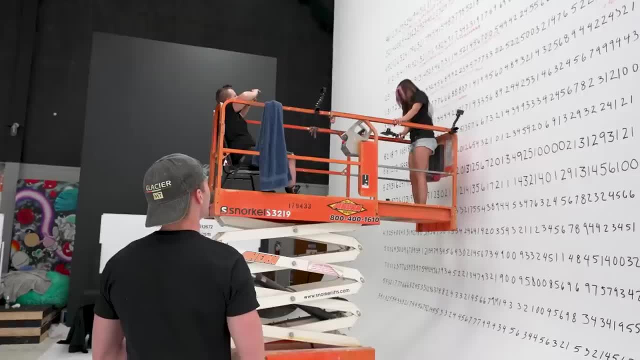 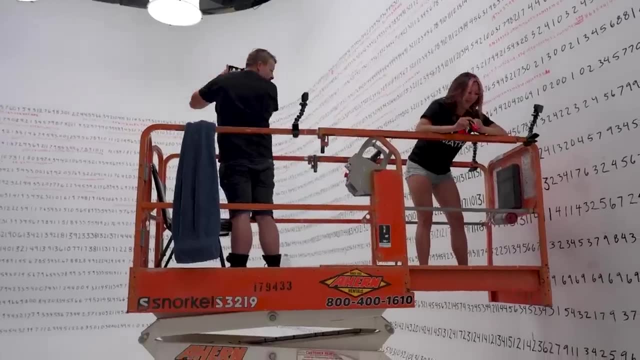 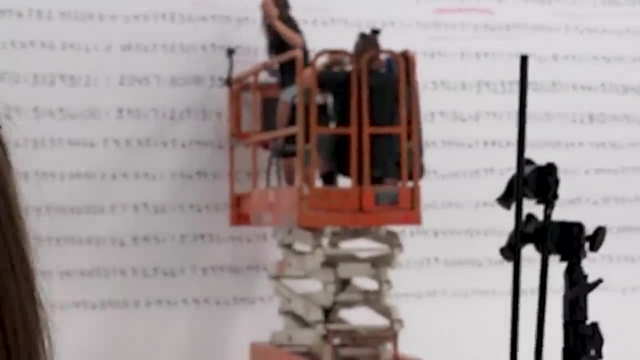 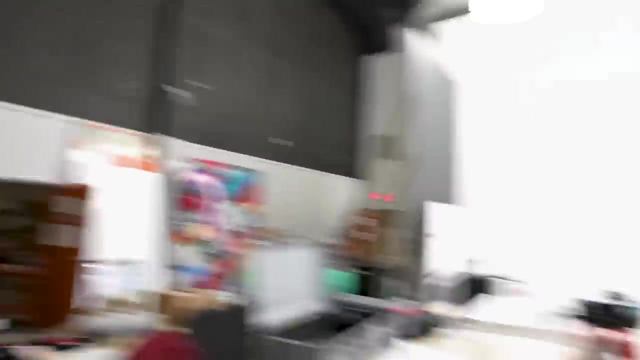 And I'm pretty proud of that. You hit my coochies. My confidence is slowly going down again. Oh, Don't Curry Curry, Curry, Heat check, Dang it. Now people are just throwing water balloons When I'm not even getting it wrong. I don't want to do this anymore. 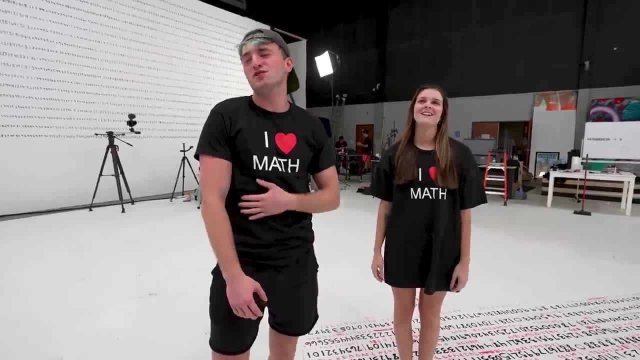 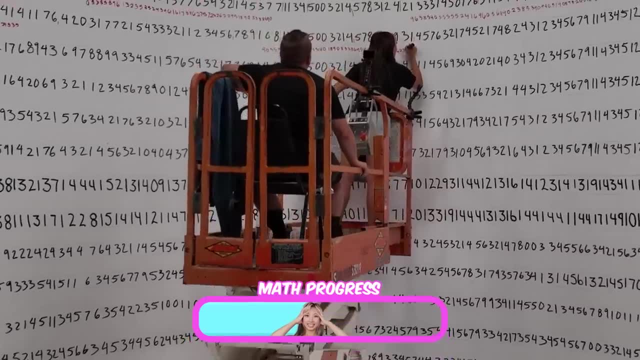 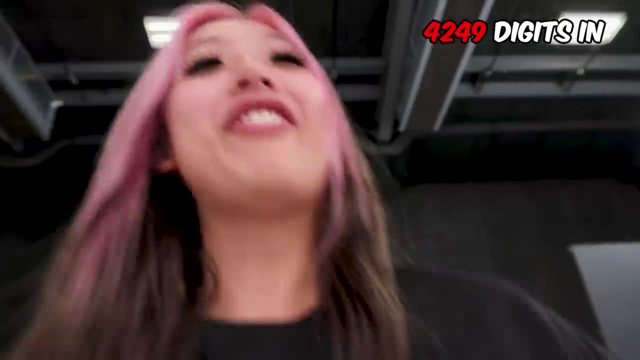 This is too hard. I can hear my friends in the background trying to cheer me up. Michelle's challenge To solve this 10,000 digit math problem Is absolutely insane, But I know that she can pull through And finish this problem. I am finally ready to get off the scissor lift. 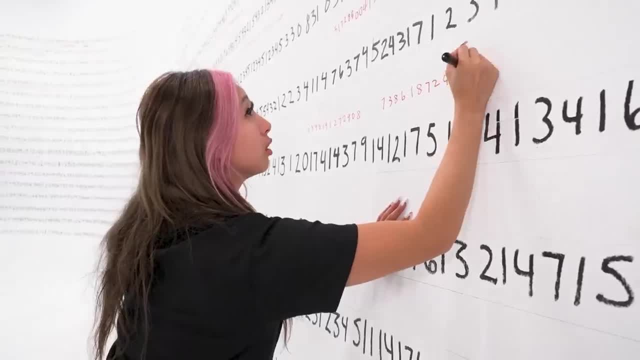 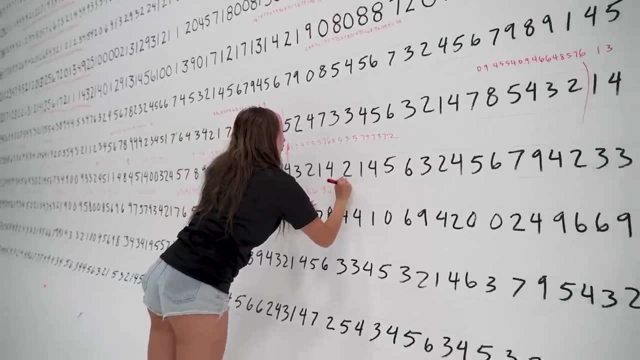 Now that I'm on the floor, I'm going much faster. It also makes my brain hurt a lot more And I'm making a lot more mistakes. Michelle seems to have everything under control, But I still kind of feel bad that she's had to do all of this. 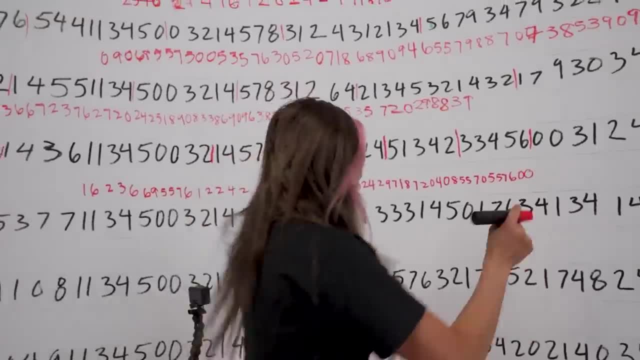 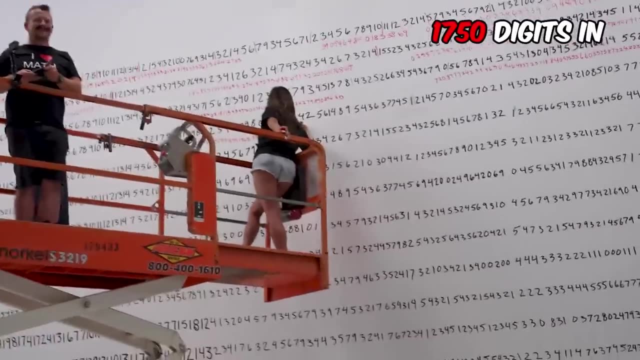 My brain is getting a little fried. Not going to lie: Zero, Zero. Kind of tired of hearing the scissors lift too. I'm not even halfway done Or even a quarter of the way done. Nine six, five, No. 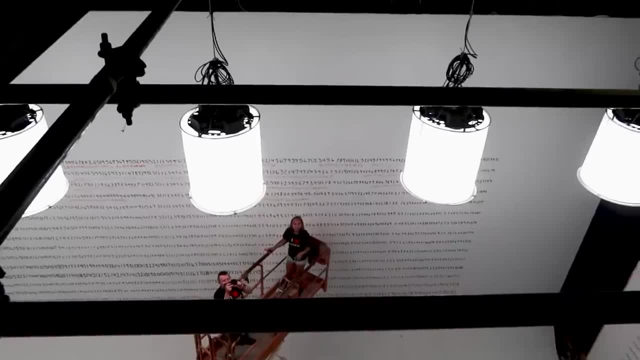 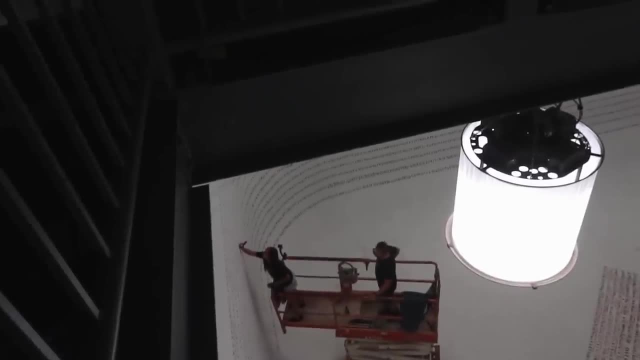 Six, six. No, I caught it before anyone else did. No one cares. Ah, Oh, It's fine, It's waterproof. Mackenzie, If you look closely, you will see a Miss Munchie in her natural habitat. 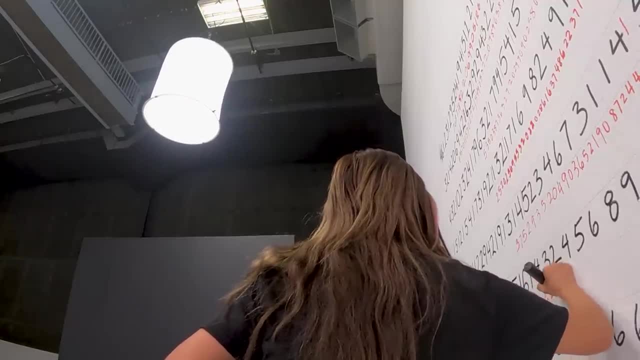 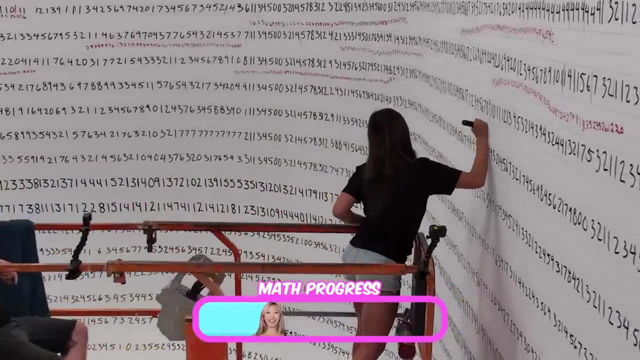 Only few species will tackle a problem. this big Thanks for watching Animal Planet, Currently six rows in. I don't think I feel confident about finishing by six hours, but I do feel confident about finishing the whole thing. So far I've only got like four wrong and I'm pretty proud of that. 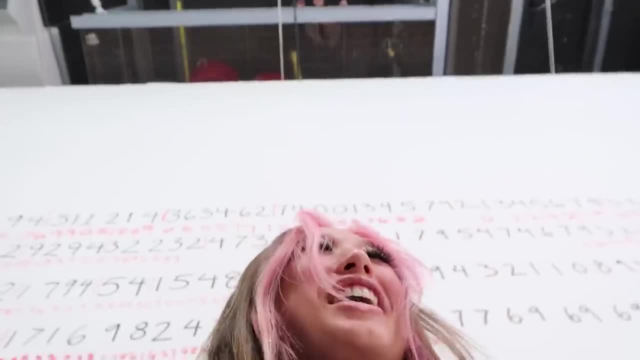 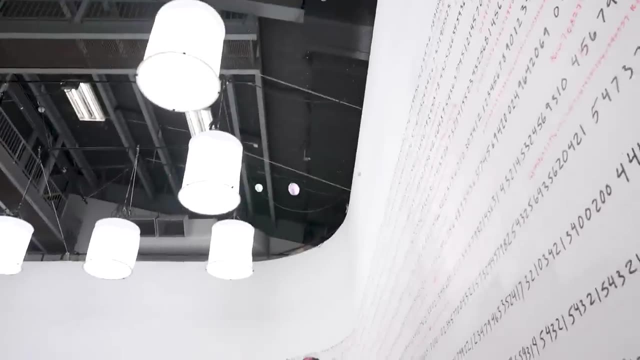 Oh, Oh Oh. You hit my coochies. My confidence is low. My confidence is slowly going down again. Oh Don't, Oh, Curry, Curry, Curry, Oh, Heat check, Dang it. Now people are just throwing water balloons when I'm not even getting it wrong. 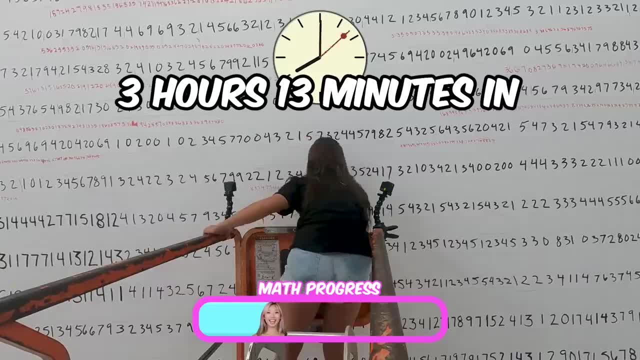 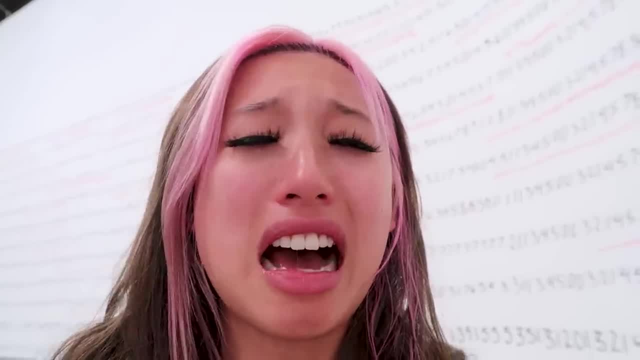 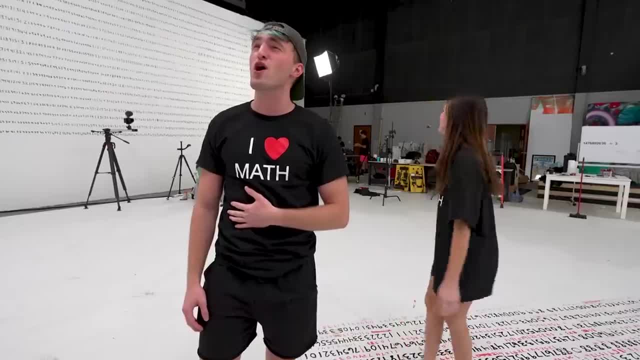 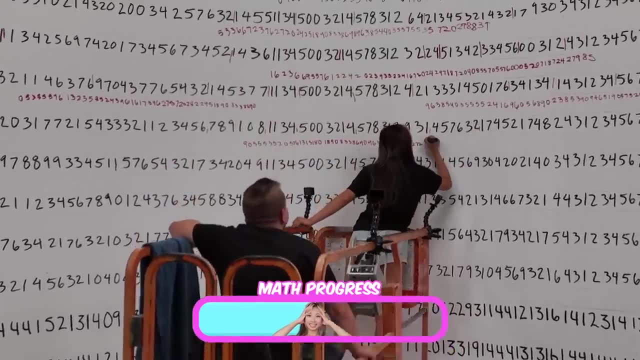 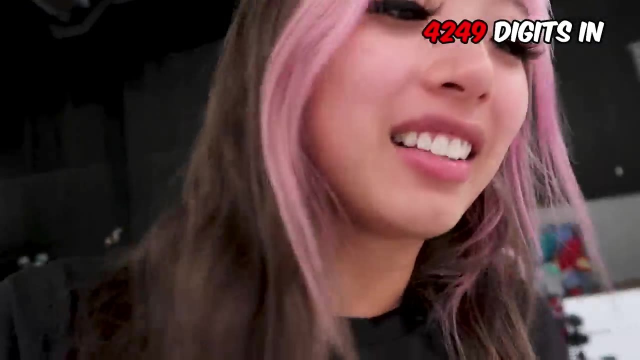 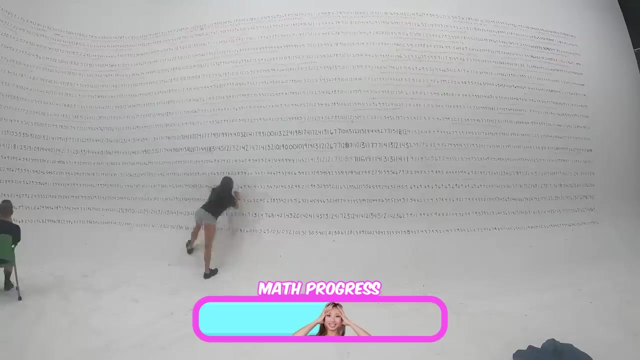 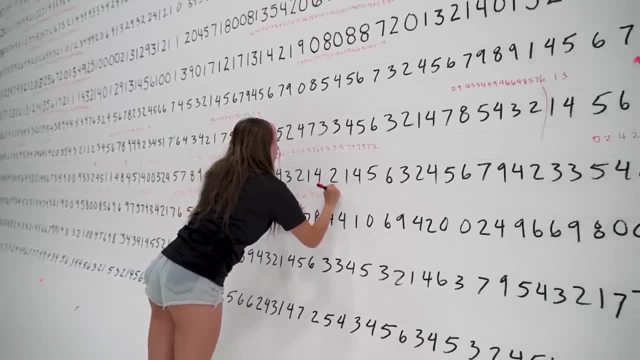 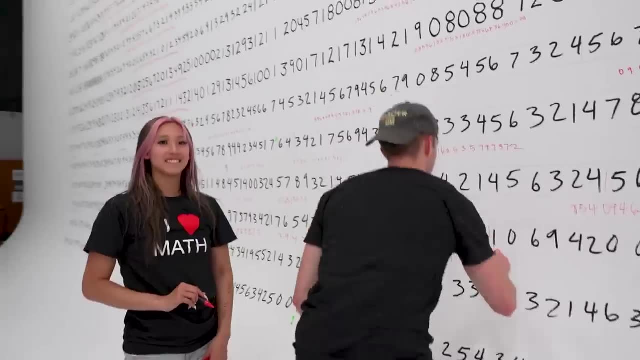 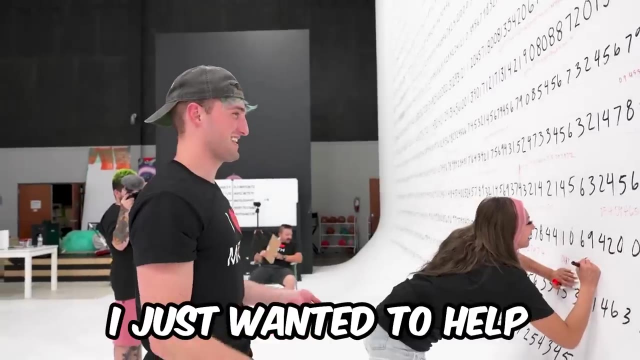 Oh, Oh, Oh, Oh, Oh, Oh herself. so i'm gonna offer some help. stop right there, oh, thank goodness. is this a two? no, is it a four, no, five, i don't think you're gonna get it. six, no, nine, no, i just wanted to help. five, five. 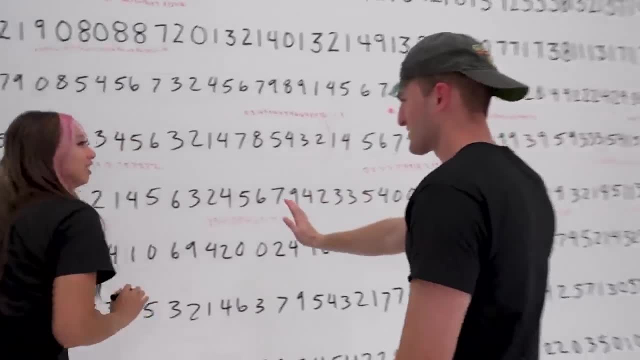 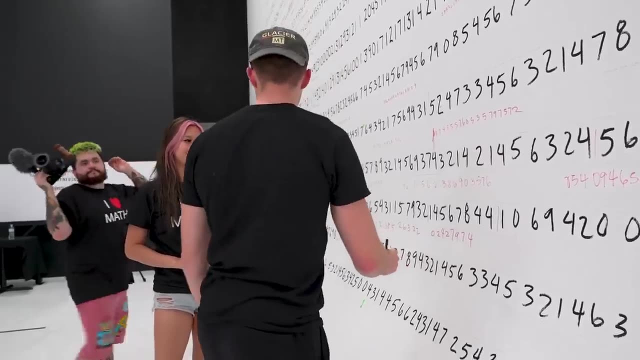 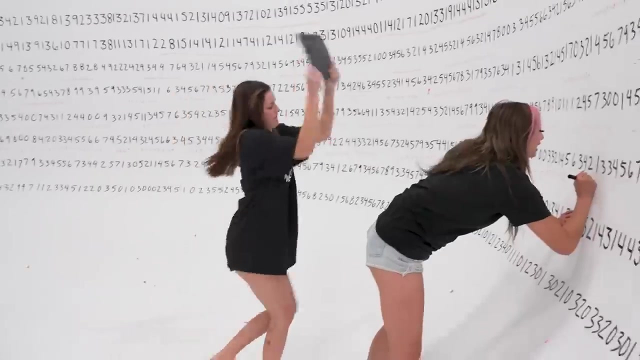 By herself. So I'm going to offer some help. Stop right there. Oh, thank goodness. Is this a two? No, Is it a four? No, Five. I don't think you're going to get it. Six, No, Nine, No, I just wanted to help. Five, Five, Three. 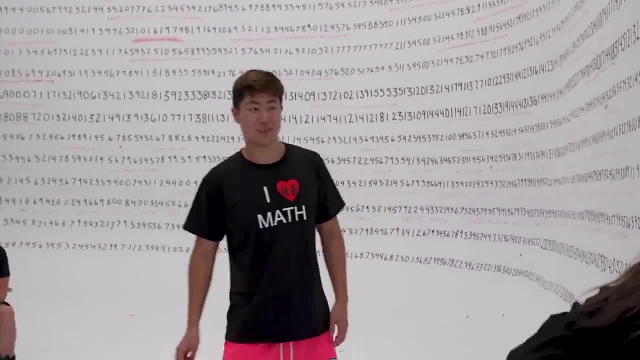 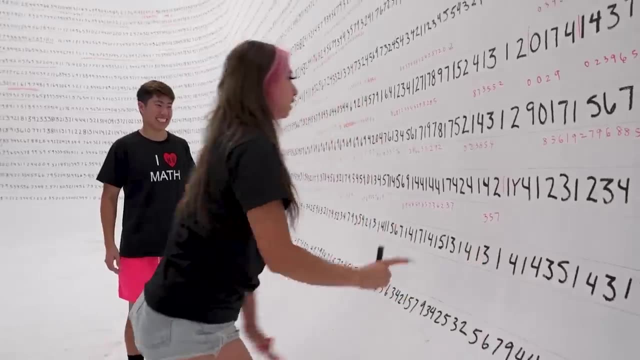 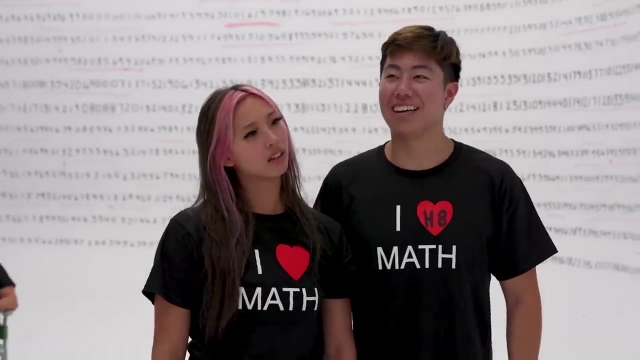 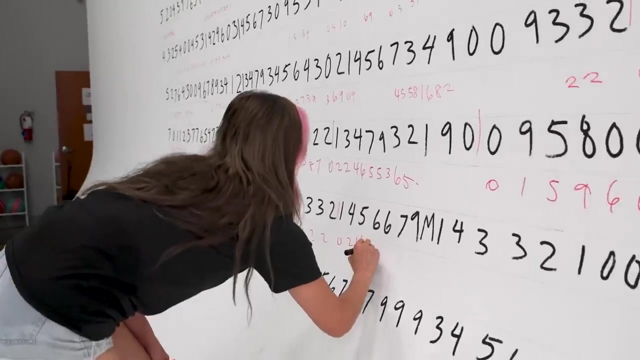 Five, Seven, Six. I got you water. That actually helped a lot better than Jake's. I'm more useful. I need a nap. Four Zero, Nine, Three, Nine, Three, Eight, Five, I need a nap. I just added a random letter, You messed me up. Three, Two, Two, Nine, Two. 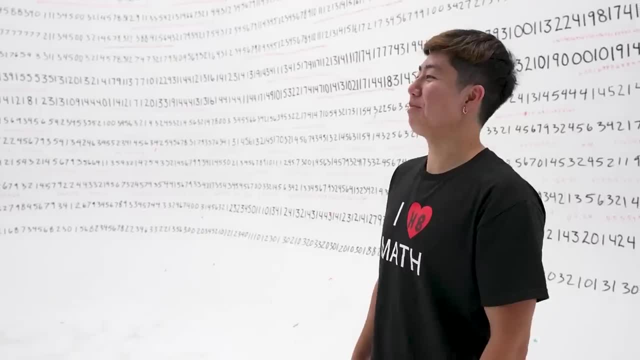 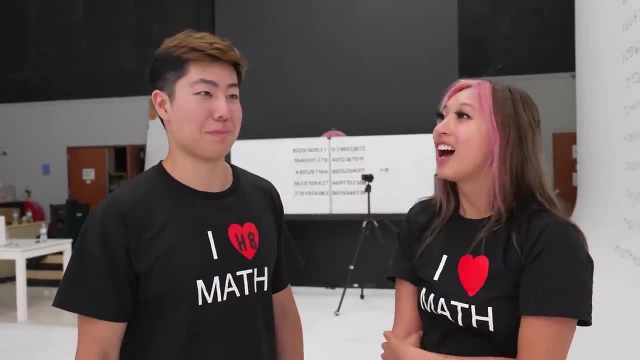 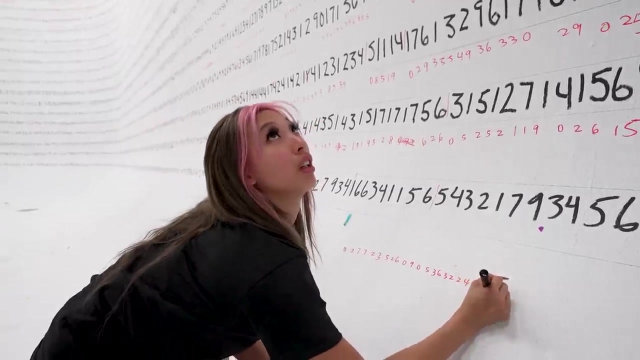 Seven Seven Nine. So it replies to an M, M for Michelle. Also, when writing out these numbers, Your phone number is somewhere on this wall, In case anyone wants to try to find it. Currently on the last row, My brain is so tired. Seven, Okay, I'm ready to go up there. 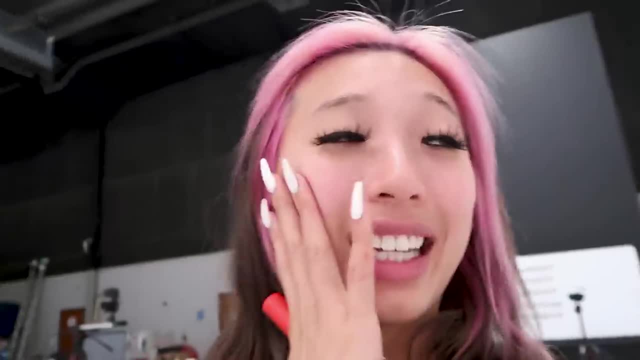 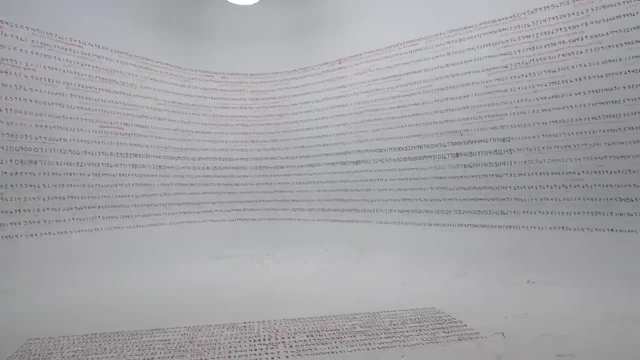 I'm five hours and forty-two minutes in, But I still have a whole other wall left. But I finished this entire wall, Which I'm very proud of myself, for I think this just shows how insane Michelle's problem is, Because just writing out like random numbers on this wall 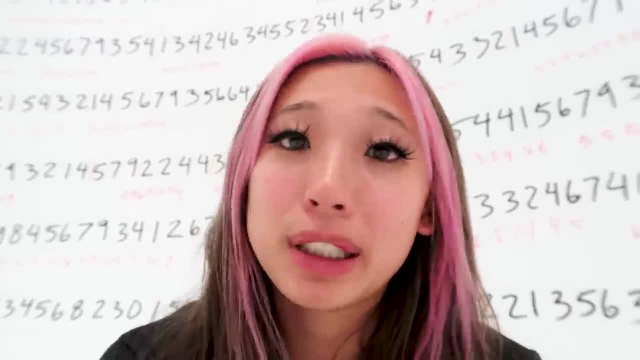 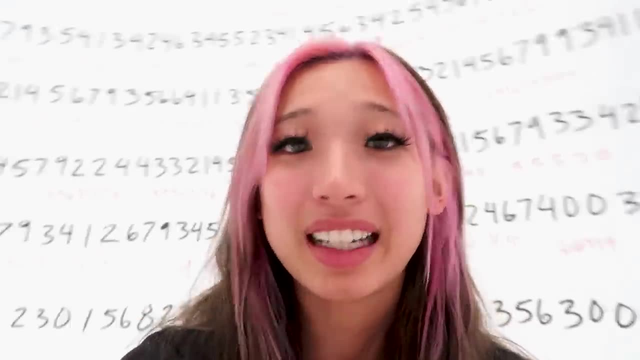 Was already super difficult. I know a lot of you guys might be struggling in your own math classes. Growing up, I also struggled a lot too. I'm here to tell you: don't give up, Keep pushing. I'm here to support you and I hope you find this video inspirational. 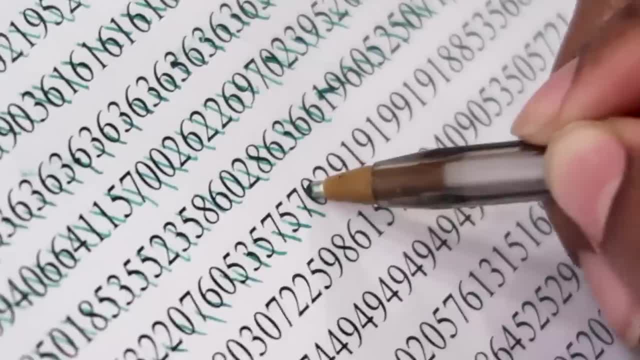 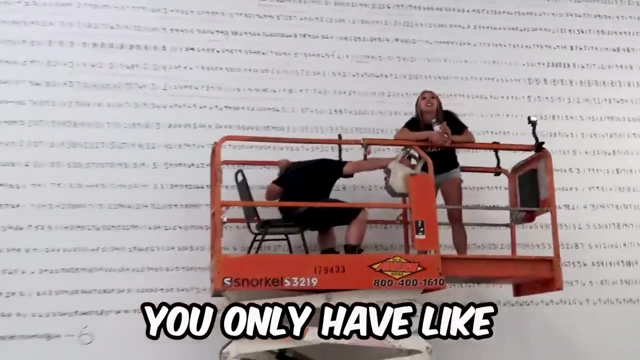 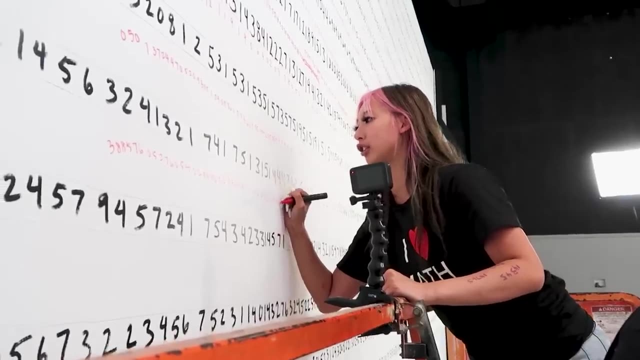 Three, Five, Seven, Five Seven Zero Two Nine Arm is cramping. Go Michelle. You only have like a thousand digits left. She's like nine thousand digits in And she's still solving it like it's nothing. It's so crazy how much I've done. I never thought that I would be able to do a ten thousand digit math problem. 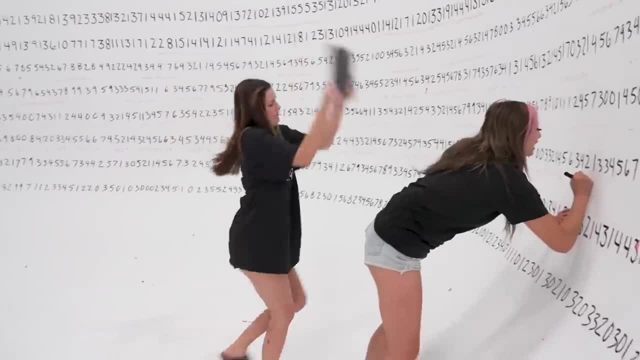 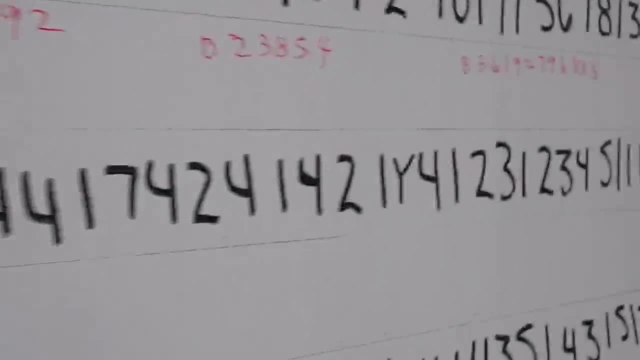 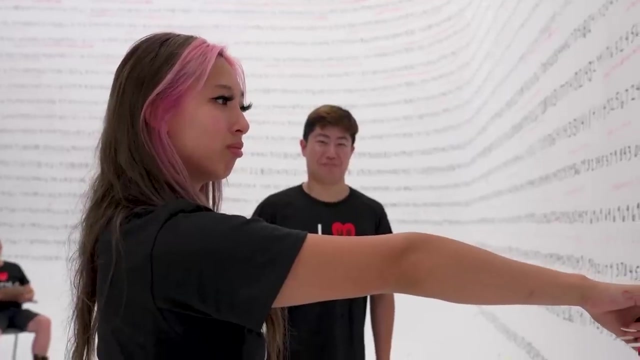 three, five, seven, six. i got you water that actually helped a lot better than jake's. i'm more useful. i need a nap. four zero, nine, three, nine, three, eight, five, three, five, seven. why is there a y? oh, i thought it was like an eight. that's an eight. did you do that? i just added a random letter. 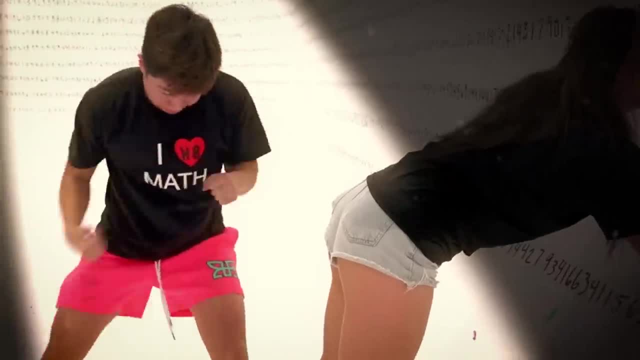 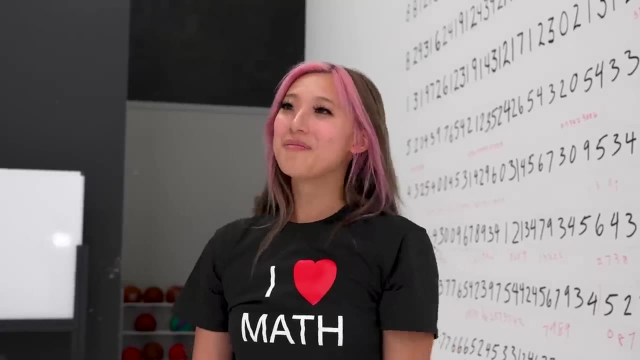 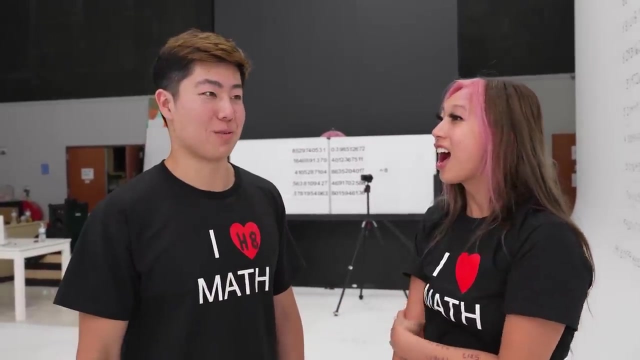 you messed me up. two, nine, two, seven, seven, nine, is that right? why is it an m? m for michelle? oh, also, when writing out these numbers, your phone number is somewhere on this wall, in case anyone wants to try to find it. currently on the last row. my brain is so tired. 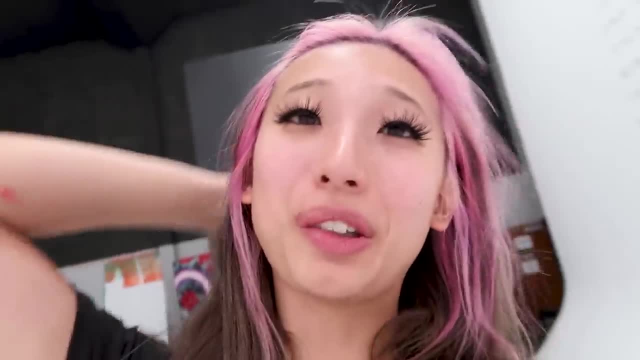 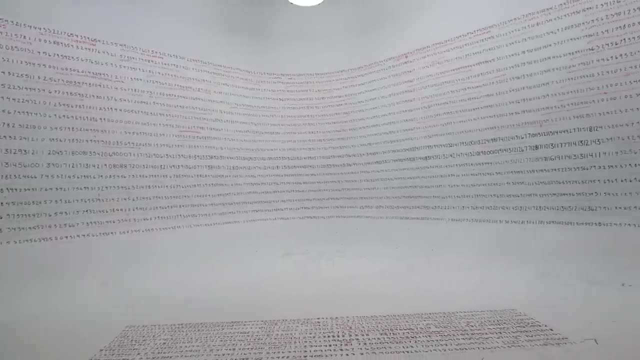 okay, ready to go up there. i'm five hours and 42 minutes in, but i still have a whole another wall left. but i finished this entire wall, which i'm very proud of myself, for i think this just shows how insane michelle's problem is, because just writing out like random numbers 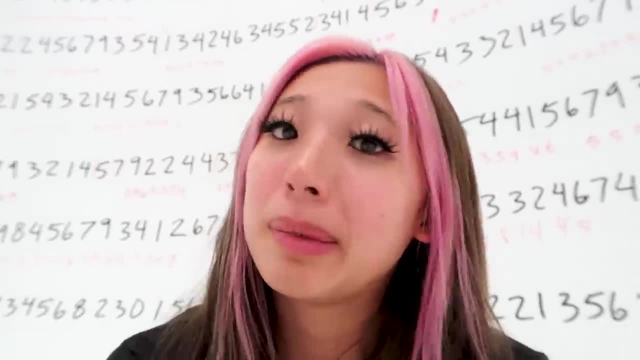 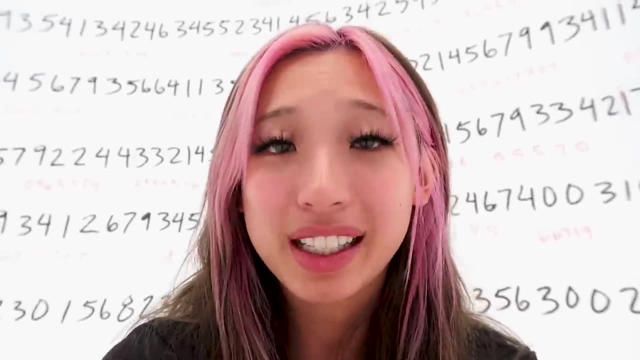 on this wall was already super difficult. i know a lot of you guys might be struggling your own math classes, so in up, i also struggled a lot too. i'm here to tell you: don't give up, keep pushing. i'm here to support you and i hope you find this. 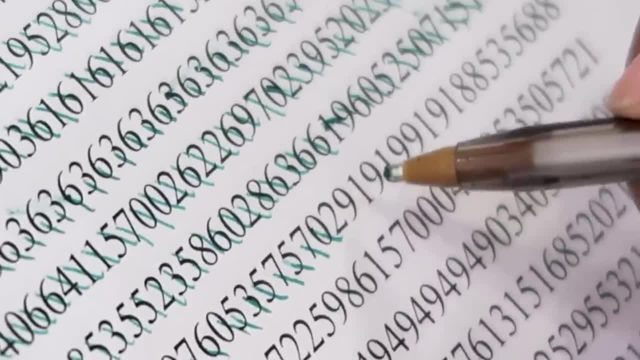 video inspirational: three, five, seven, five, seven, zero, two, nine arm. it's cramping. go, michelle. you only have like a thousand digits left. she's like 9 000 digits in and she's still four, six and 3, 6, seven, seven, six h�. 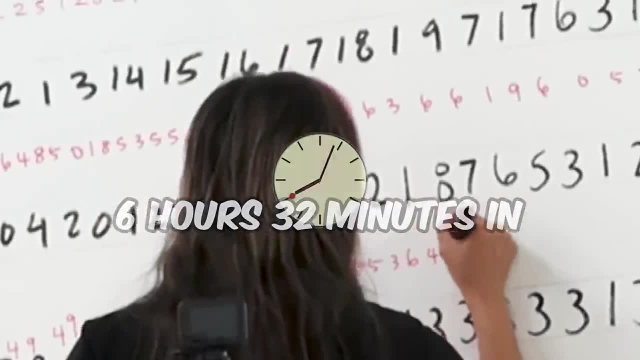 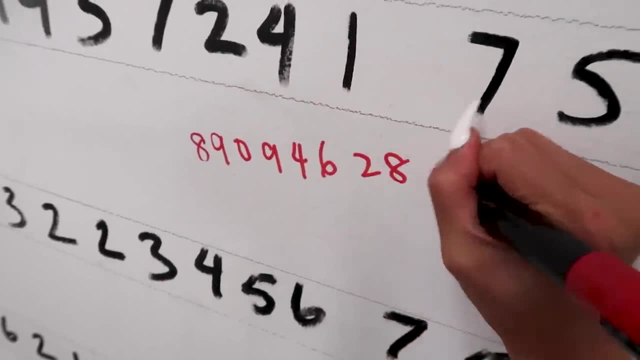 whoops, I mean, that's true, Solving it like it's nothing. It's so crazy how much I've done. I've never thought that I would be able to do a 10,000 digit math problem. It's definitely been a real challenge today. 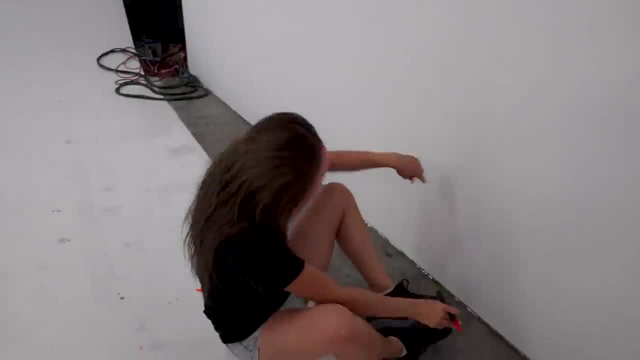 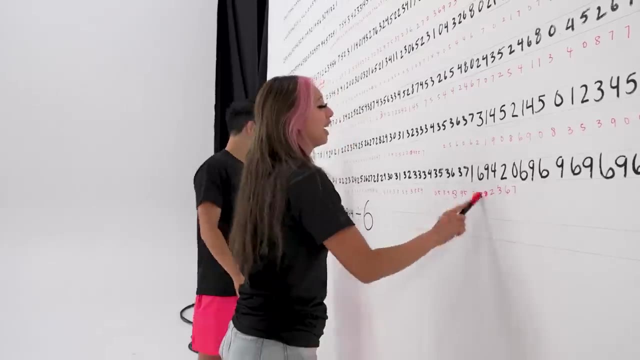 six, seven. You're almost there, Michelle, Michael, You're almost there, Come on. Come on, My brain is messed up. You've done all of this like you only have this: Okay, eight, eight, two, three, six, seven, eight, seven. Last line, Last line. 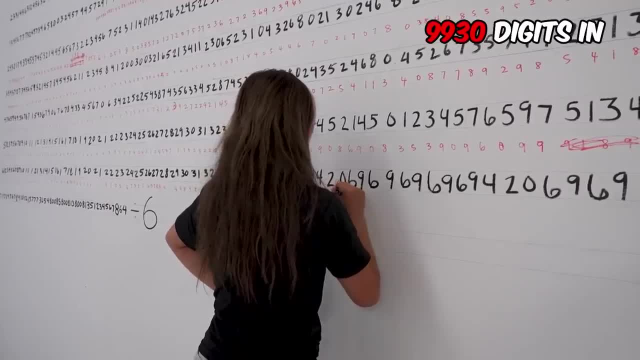 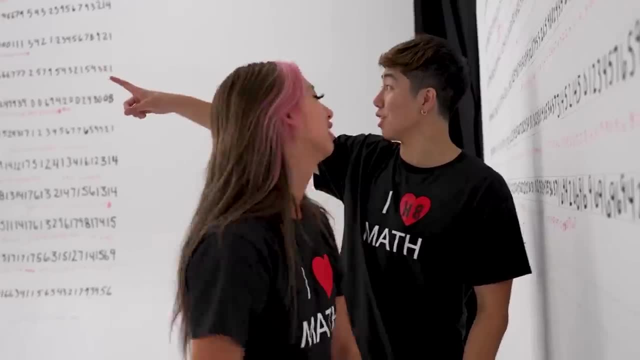 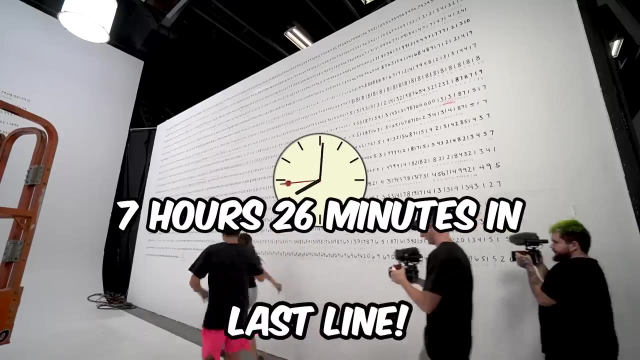 It's definitely been a real challenge today. Six, Seven, Ugh, You're almost there, Michelle, Michael, you're almost there. Come on, You're almost done. My brain is messed up. You've done all of this Like. you only have this. Okay, Eight, Eight, Two, Three, Six, Seven.